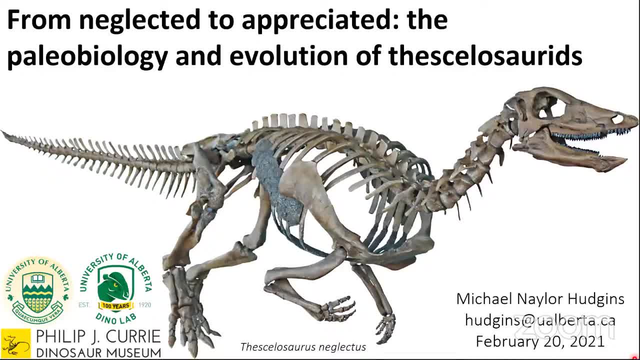 Hello, Welcome to the Philip J Currie Dinosaur Museum Virtual Speaker Series, where we have paleontology guests call in for a presentation on science, fossils and dinosaurs and where the public will be able to ask questions live on YouTube. First off, we want to acknowledge that we are on the homeland of the many diverse First Nations. 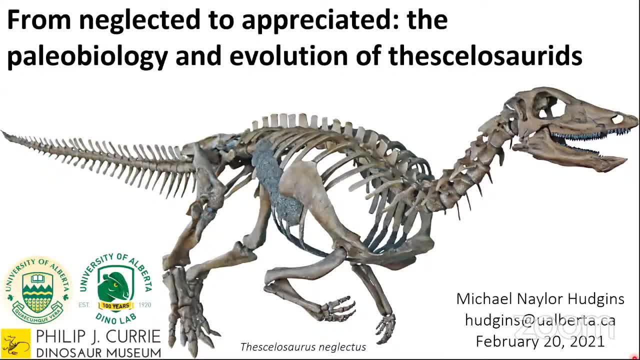 and Métis, people whose ancestors have walked this land since time immemorial. We are grateful to work, live and learn on the traditional territory of Treaty 8.. Today, Michael Hudgens will be presenting his talk titled From Neglected to Appreciated: The Paleobiology and Evolution. 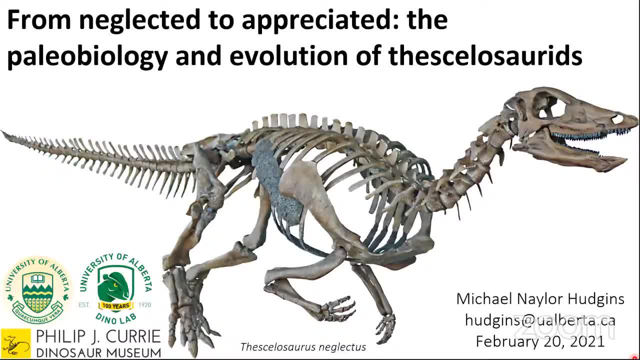 of Thesilosaurids. Michael is from Yorktown, Virginia, which is three hours south of Washington DC. Growing up, Michael was captivated about the natural world, including rocks and extinct animals. Although his interest about the natural world wavered throughout life, he ultimately 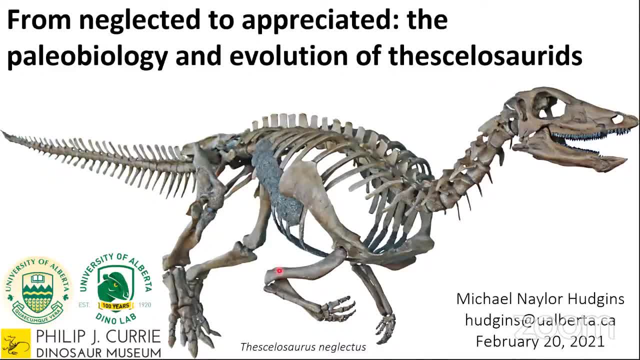 pursued and completed his undergraduate degree in geology at George Mason University in Fairfax, Virginia. Michael then went on to pursue his master's in evolutionary biology at the University of Alberta in Edmonton, supervised by Dr Corwin Sullivan. He is currently writing his master's. 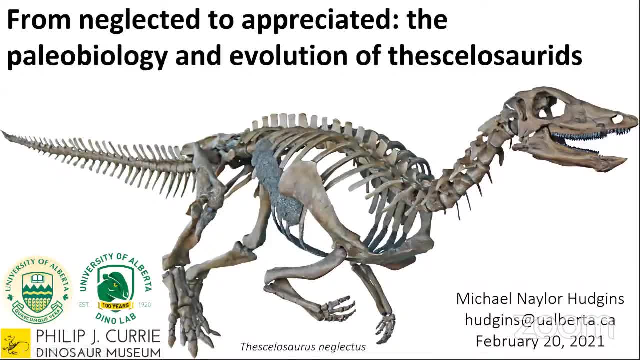 thesis on Thesilosaurids from northern and southern Alberta. For those turning in, you can type your questions in the comments section and I'll read them to our speaker at the end of the talk. Thank you for joining us today, Michael, and with that I will let you take it away. 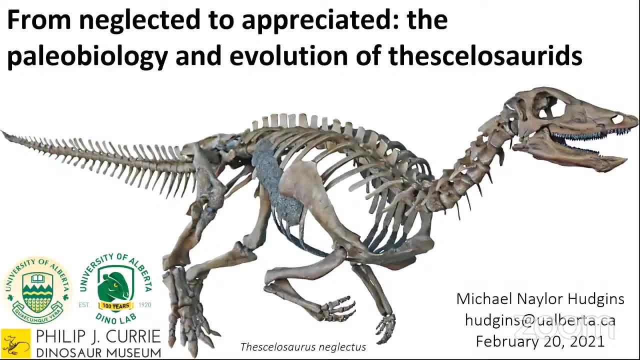 Thank you for that kind introduction. So today we're going to be talking about the paleobiology and the evolution of Thesilosaurids and I'm going to be briefly talking about some of the new material coming out of the DC bone bed in Wembley. excuse me, 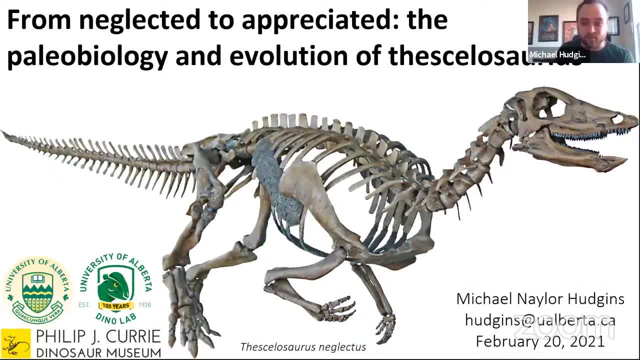 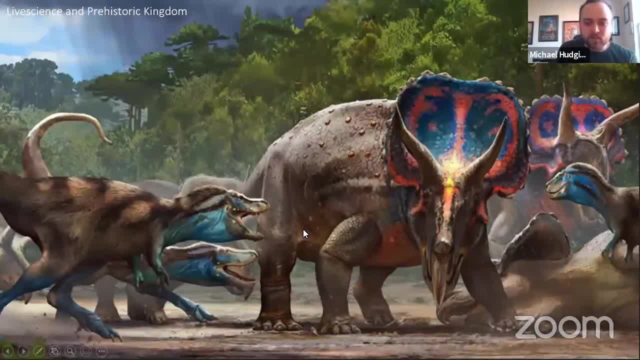 in Grand Prairie, Alberta, just up the street from Philip J Currie Dinosaur Museum. So most people don't realize that a lot of these dinosaur-dominated ecosystems during the late Cretaceous period were dominated, not dominated they were, that there were other organisms that. 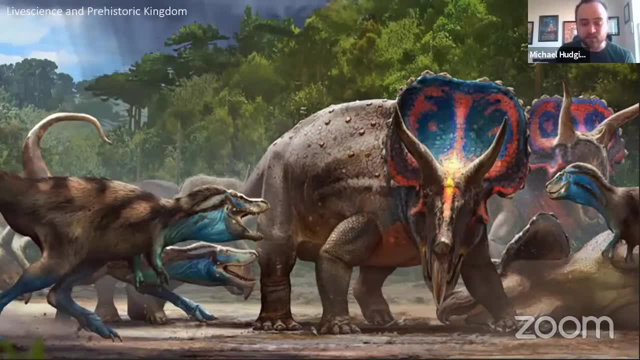 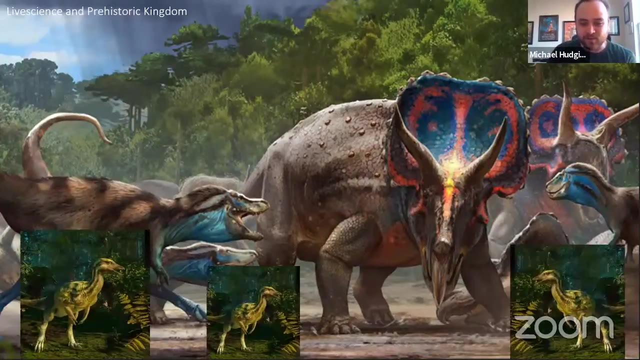 were not gigantic animals such as like Triceratops and Tyrannosaurus rex, as well as Edmontosaurus. This includes small-bodied Ornithischian taxa, which would be making, which would be made up majority of Thesilosaurid taxa, So a good representation would be Thesilosaurids. 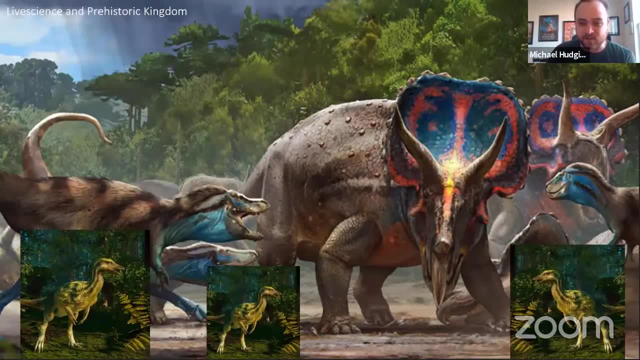 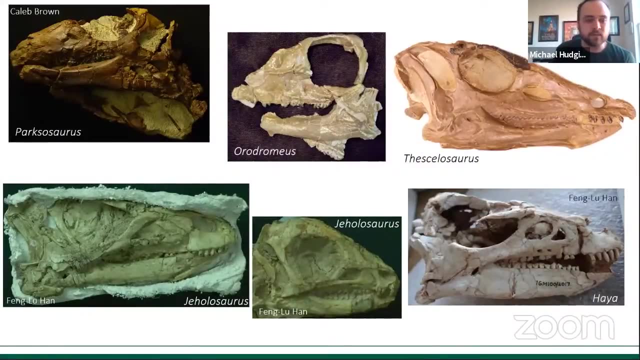 running around with these gigantic Ceratopsid and Trinosaurid-type animals during the late Cretaceous period, And so these Thesilosaurid taxa are quite diverse during the late Cretaceous period, such as Parxosaurus, Orodromius, Thesosaurus and Haya and Jeholosaurus may be a little contentious about. 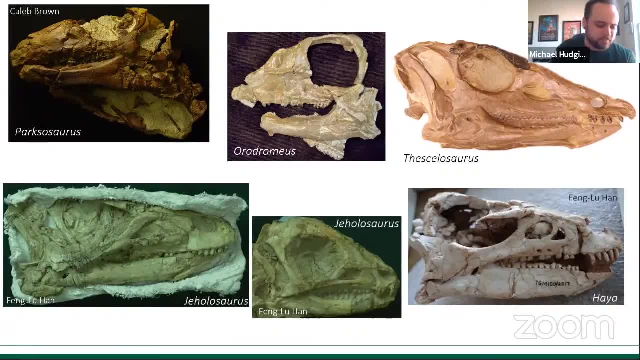 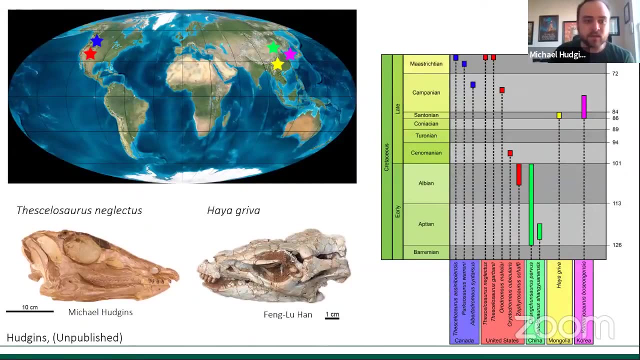 its placement in Thesosaurids. as they are, their phylogenetics, their evolutionary histories place them sometimes within Thesilosaurids and sometimes with outside of Thesilosaurids, And so the biogeography of Thesilosaurids during the late Cretaceous. we only know, we only. 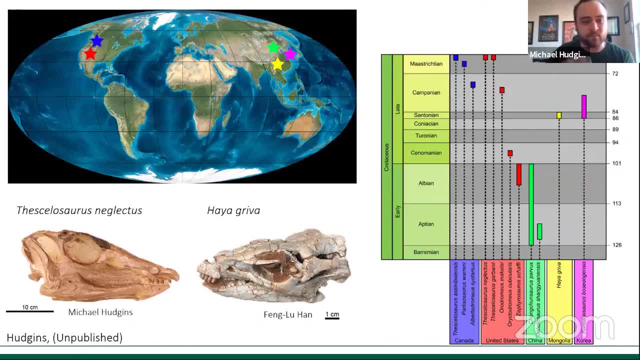 recovered a few fossils from. we recover fossils from North America as well as in Asia, So North American taxa are both found in Canada and in the United States and this includes, like Thesilosaurus neglectus, Parxosaurus, Albertodromius, Orodromius Zephyrosaurus and Arachnoptera. 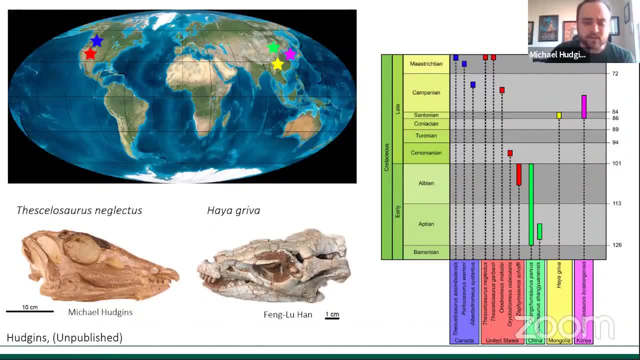 And Asian taxa are represented by Haya, which is found in Mongolia, Changchunosaurus, which is found in Asia, and Jeholosaurus, which is a potential Thesilosaurid that is found in China as well as Korea, with Crianosaurus, As you see here by this graph. 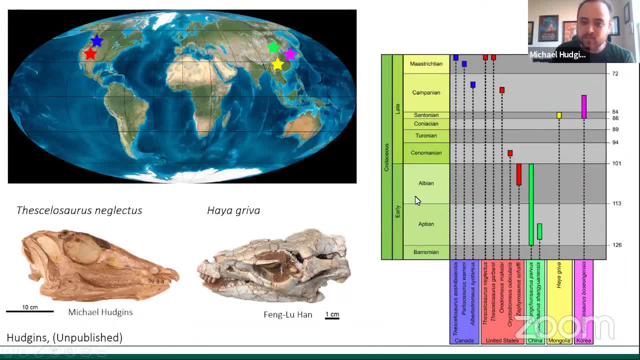 there is a, the Cretaceous time scale, with the oldest at the bottom and the Mastrichtine at the top, which is coinciding with the end of the dinosaurs, which is further closer to the present, And you can see that Canada has specimens here, which is by Thesilosaurus acinoboensis. 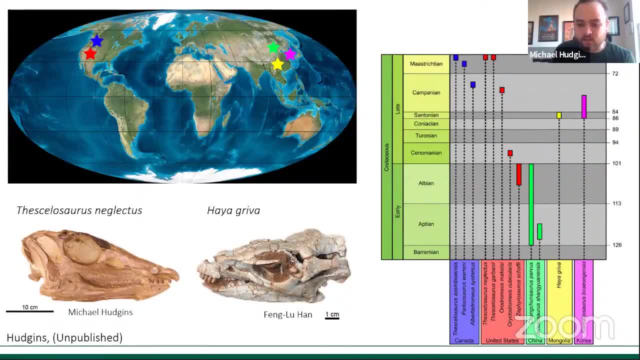 Thesilosaurus neglectus, Parxosaurus, and the United States with Thesilosaurus neglectus and Orodromius, as well as China specimens, Mongolian specimens and Korean specimens. And we have two skulls, Thesilosaurus neglectus from North America and Haya from Mongolia. 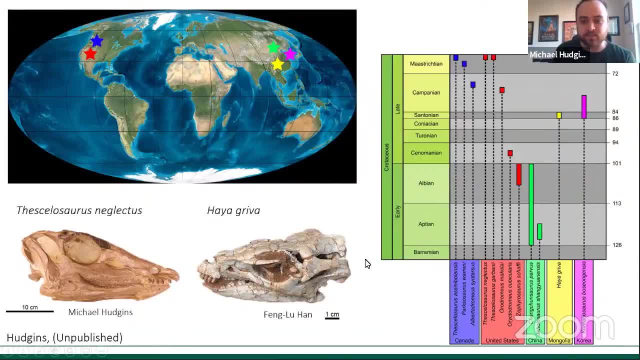 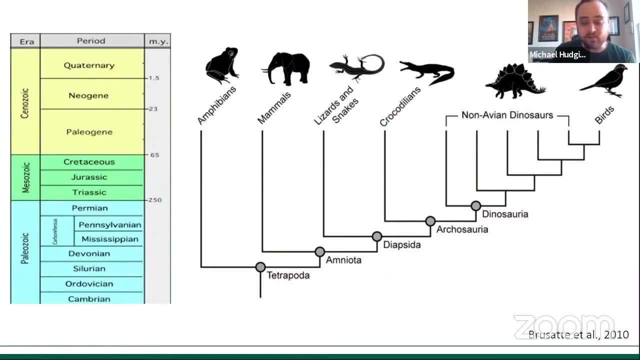 which are representative of North American taxa And an Asian taxa. So I'm going to talk about the phylogeny of dinosaurs and where Thesilosaurids are placed within Dinosauria. So here is a simplified phylogeny of tetrapod organisms that live. 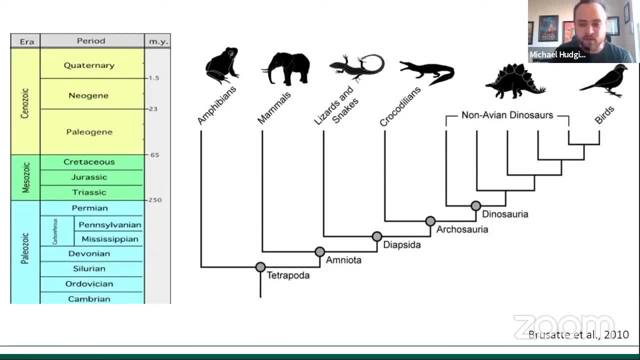 on planet Earth. We have amphibians, mammals, lizards and snakes, crocodiles, non-avian dinosaurs and birds. On the left we have the geological time scale, with at the bottom again is the oldest And at the top is present day. 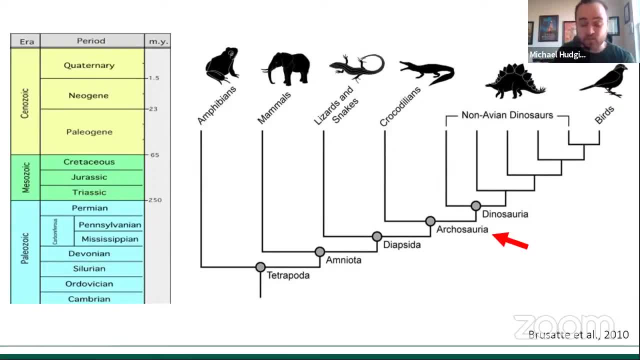 So dinosaurs are unique, are placed within a unique clade of organisms called archosauria, which includes crocodilians and as well as birds, And birds are within, as you see, with Dinosauria. So there are avian dinosaurs and the non-avian dinosaurs which are your Stegosaurus. 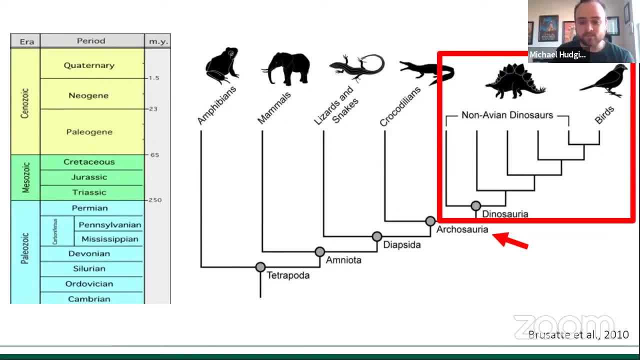 your Tyrannosaurus rex, your Triceratops and as well as your Thesilosaurids And dinosaurs live in a time period called the Mesozoic, And the Mesozoic is broken down into three sections. You have the Cretaceous, the Jurassic and the Triassic, And Thesilosaurid taxa are usually found. 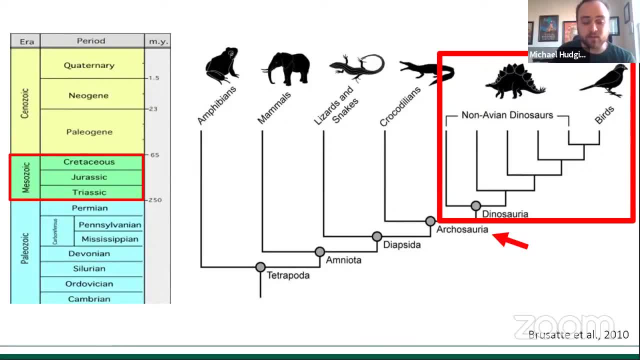 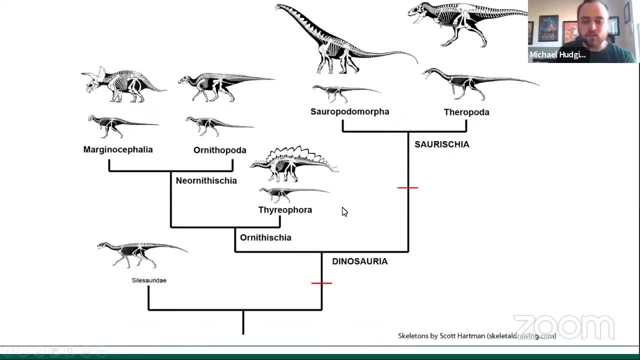 or mostly found in Cretaceous, in the Cretaceous time period, closer to the upper part of the Cretaceous, towards the end of the dinosaurs. So getting a closer resolution of dinosaur phylogeny. dinosaurs can be broken down into two groups. You have Saurischians and then you have 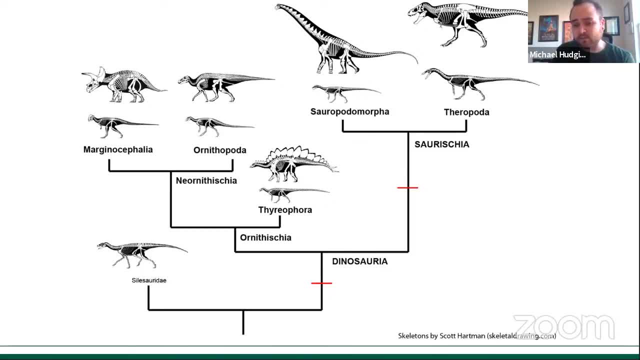 Ornithischians. Saurischians can be broken down further into Theropoda and Sauropodomorpha. Theropoda, which includes your Tyrannosaurus rex, your Velociraptor, as well as birds, And Sauropodomorphs are your long-necked dinosaurs in the late Jurassic and also the Cretaceous period. 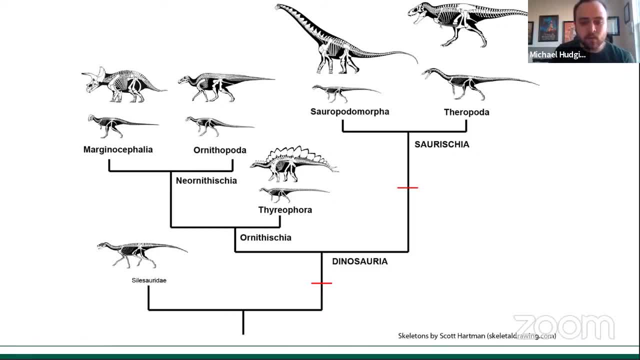 the really gargantuan animals. Ornithischians can be broken down into three groups, which would be Thyrirphorians, which are your Stegosaurus, your Ankylosaurids, as well as your Ornithopods, or their own group, which we'll be discussing. 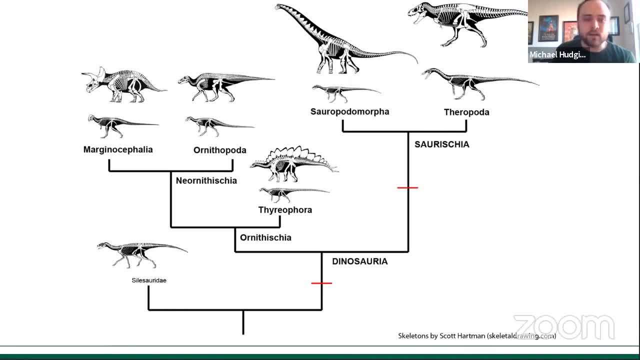 further. This is where Thesilosaurids are thought to be present in, and Edmontosaurus are within, Ornithopod groups in Ornithopoda. And then, lastly, Ornithischians can be broken down into Marginal Cephalians, which includes your Pachycephalosaurids and your Triceratops. 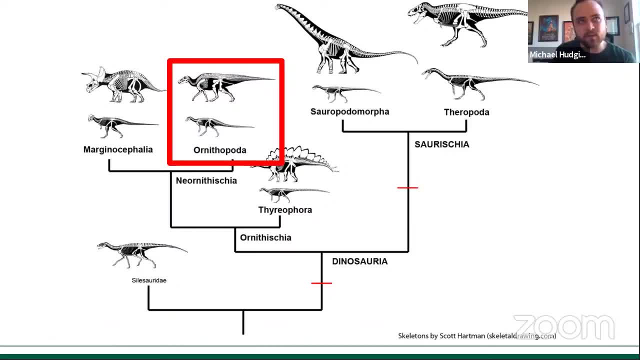 So Ornithopods with Thesilosaurids are. their evolutionary history is fairly contentious. We don't really know exactly where Thesilosaurids belong around the Ornithischian tree, but we have some ideas. But for the sake of this, 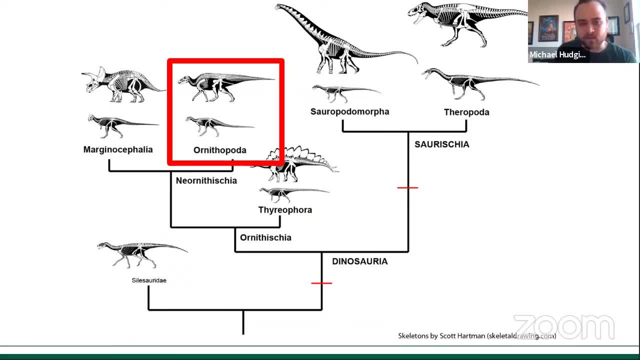 they are sometimes classified in Ornithopoda, But later on in this talk we will see that sometimes they are placed outside of Ornithopoda, And thus I will be calling them fairly basal Ornithischian taxa. And so this leads into what do I mean by basal. 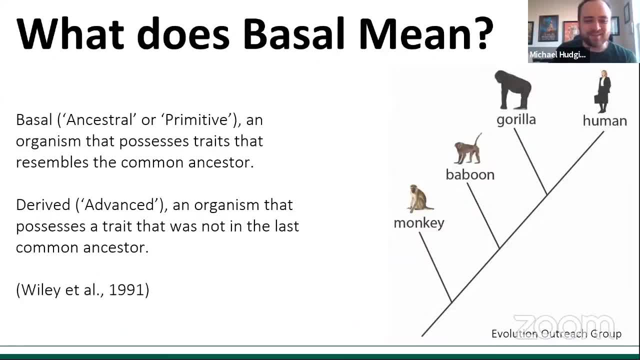 And it's not an herb, but basal- is the ancestral or primitive condition, And it's basically an organism that possesses traits that resemble the common ancestor. And the opposite of ancestral or primitive is derived, which means advanced, And it's basically an organism that possesses a trait that was not in the last common ancestor. 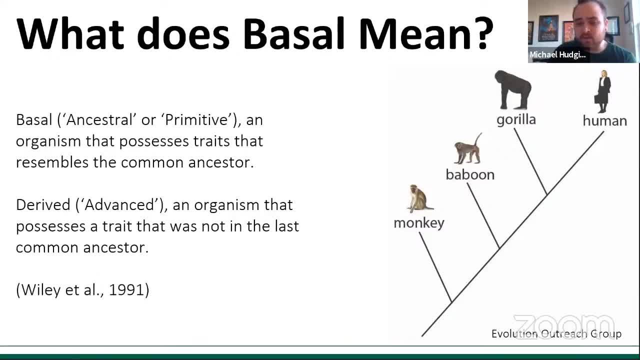 So, for an example, we had the phylogeny of primates, with humans and gorillas being more derived and monkeys and bamboos being more basal. So monkeys have a lot of characteristics that are in common with the common ancestor, that are present within the common ancestor. 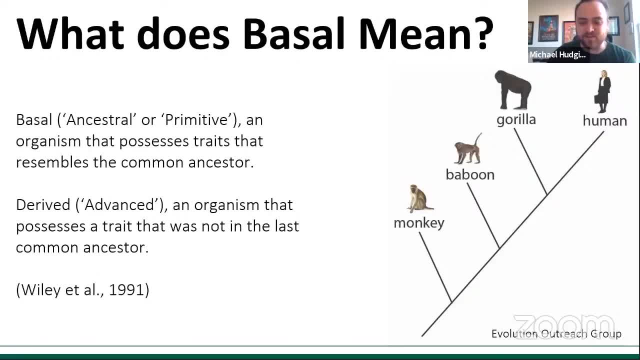 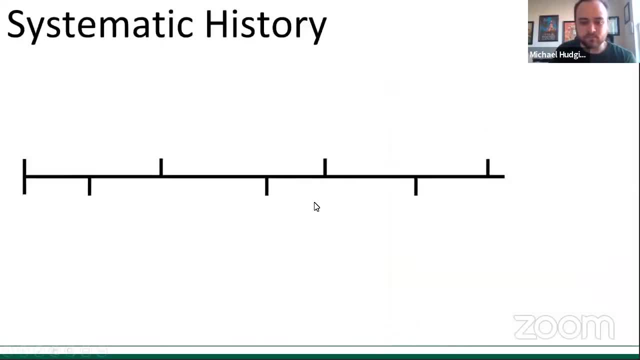 while gorillas have more derived traits, They don't have a lot of characteristics that are in common with monkeys or the common ancestor. So the systematic history, or the taxonomy of Thesilosaurids is fairly complex, And so I'm going to give a very short summary of the taxonomic history of Thesilosaurids. 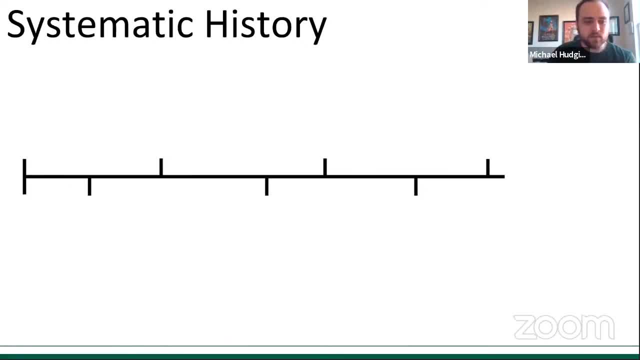 for context of this talk. So the first ever small-bodied bipedal plant-eating dinosaur was named and described in 1869 by Thomas Huxley, And he named it Hypsilophodon foxei, And like I said it was. 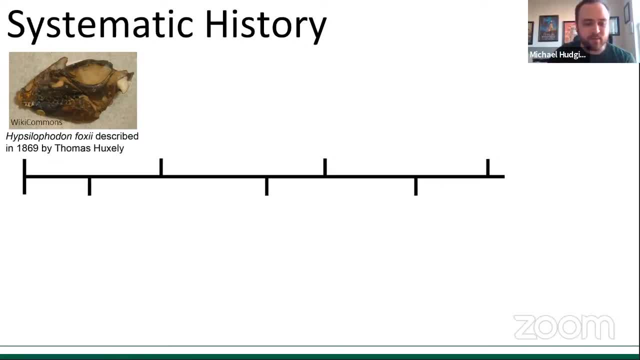 the first ever small-bodied plant-eating dinosaur. It was the first ever plant-eating bipedal dinosaur that was discovered. Hypsilophodon, during this time period, was very contentious of where it belonged in the phylogeny of Dinosauria within the taxonomy of Dinosauria, And there was a lot of heated debate. 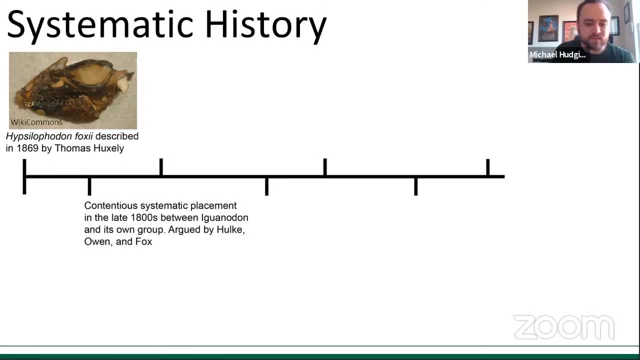 about where Hypsilophodon belonged. It was thought to be belonging at that time, thought to be belong to Iguanodons, which are larger bipedal, maybe quadrupedal, ornithischian plant-eaters. Auric made up its own group, which was argued by Hulk. 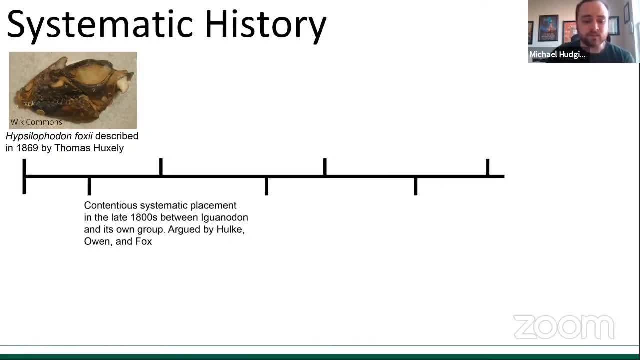 Owen and Fox during this time period in the 1800s. But Dolo in 1882, placed Hypsilophodon today in its own placement. Excuse me, placed Hypsilophodon in its own placement, called Hypsilophodon today. 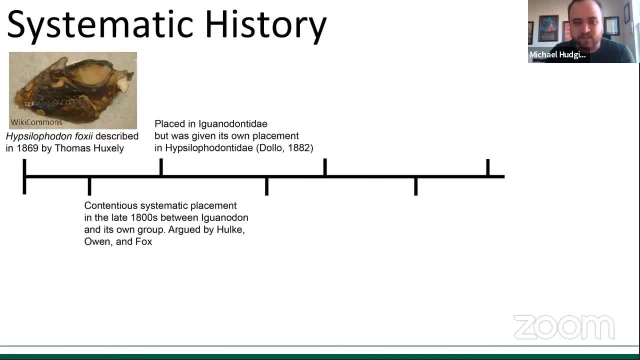 which is outside of Iguanodon today, which is the relatives of Iguanodon. Later on during the 1890s, a fossil was collected from Wyoming that was left untouched until 1910s, When a man named Charles Gilmore 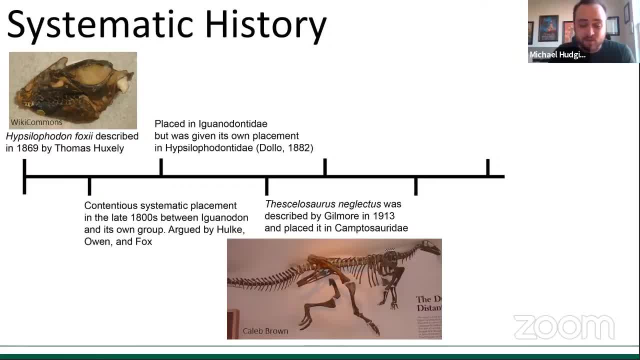 described this specimen in 1913, and he just called it Thesosaurus neglectus, which means the marvelous neglected lizard, and thus the term neglectus, And he described it in 1930 and placed it within Campsosauridae, And Campsosauridae is a late Jurassic another. 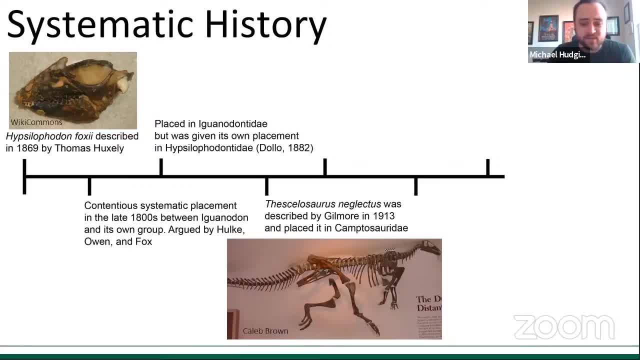 late Jurassic ornithischian that he thought at the time resembled Campsaurus. But in 1915, when he uncovered more of the fossil material, he discovered that it did not resemble Campsaurus really that much and then thus placed it within Hypsilophodon today because it resembled closely. 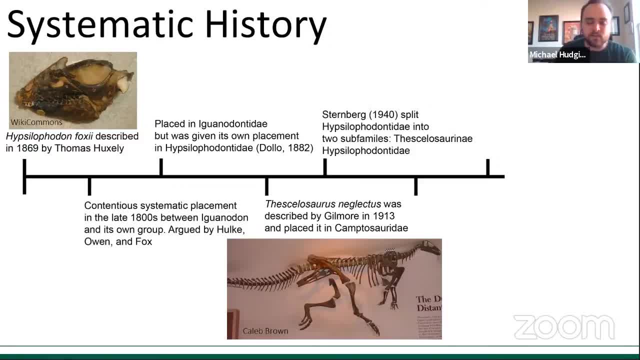 with Hypsilophodon. So in 1940, Sternberg split Hypsilophodon today into two sub-families, which is Thessalsorinae and Hypsilophodon today, which was further to discriminate the differences between Hypsilophodon and Thessalosaurus, as he discerned that there were many, many differences between the 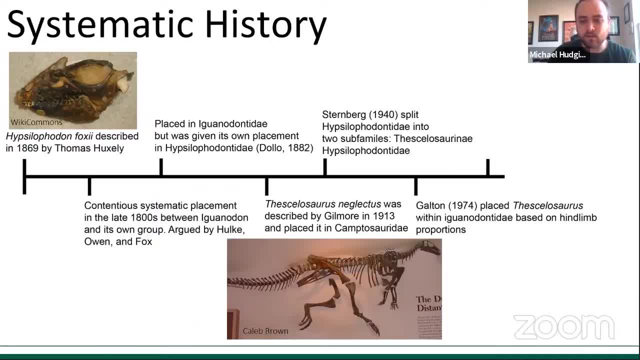 two animals. Within 1974, Galton placed Thessalosaurus within a group called Hypsilophodon, today based on Heinlein proportions. I find this as a weak argument, just basing out on Heinlein proportions, but towards the end of the 1900s and late 1900s- 1990s. 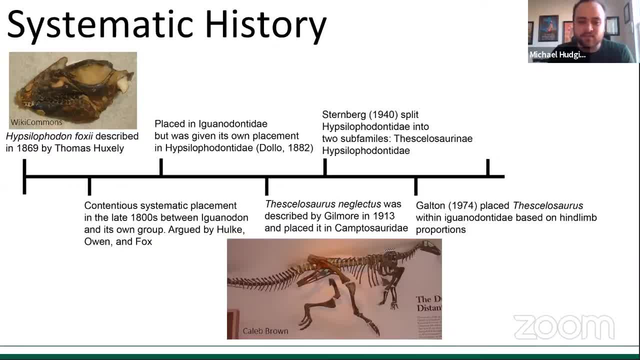 scientists have discovered that Hypsilophodon today is an invalid grouping of animals based on phylogenetic analyses And then later on, in the early 2000s, a lot more specimens of these small-bodied ornithischians, these small basal ornithischians. 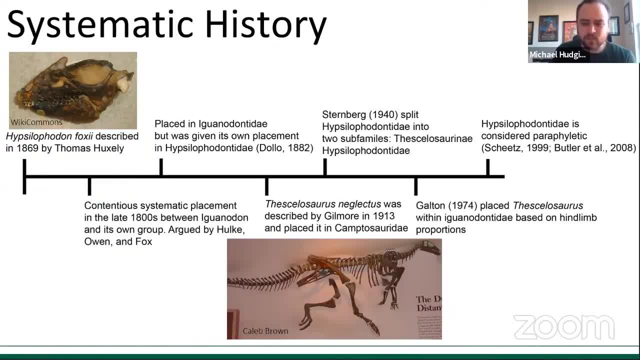 from the Cretaceous period were being recovered, and this led to a much more robust phylogenetic analysis in the early 2010s, Thus discovering or trying to figure out if there's a monophyletic group or a unifying grouping of late Cretaceous ornithischians. 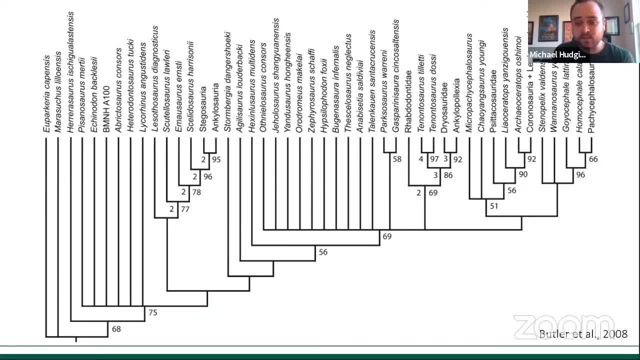 In 2008, Butler did an analysis of ornithischians in general and he recovered all the major ornithischian clades, such as marginal cephalians, ornithopods, as well as thauriophorians, But he did not get a very good resolution on Thessalosaurus neglectus and 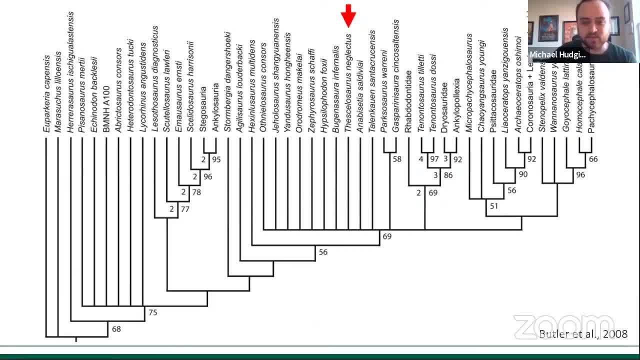 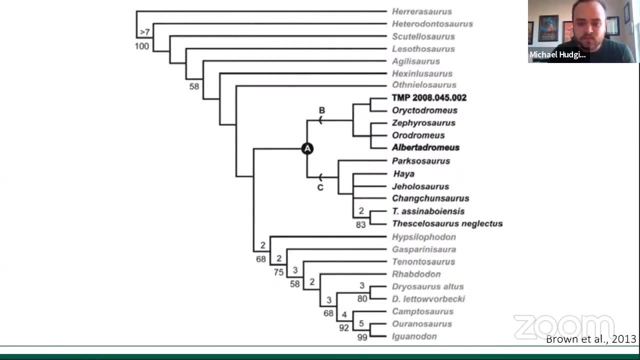 potentially closely related fossil taxa. As you see, there is a large polytomy here of unresolved evolutionary relationships Between these taxa. Later on in 2013, Brown and company tried to figure out if there's any relationships with these basal ornithischian taxa, And he did find that there was a monophyletic grouping here in node A. 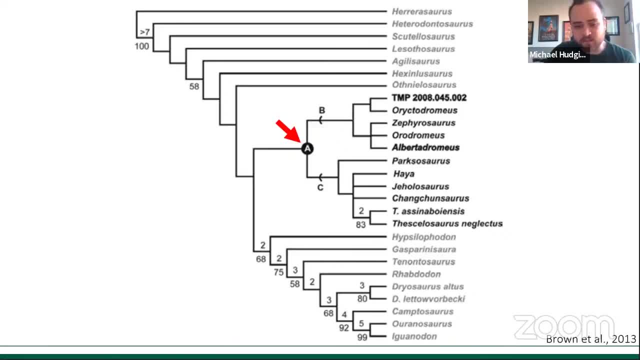 which he called Thessalosauridae, which included Thessalosaurus neglectus, Chanchonosaurus, Jeholosaurus, Parxosaurus, Orodromeus and Albertodromeus. But he also found that Thessalosauridae can be broken down into two clades. 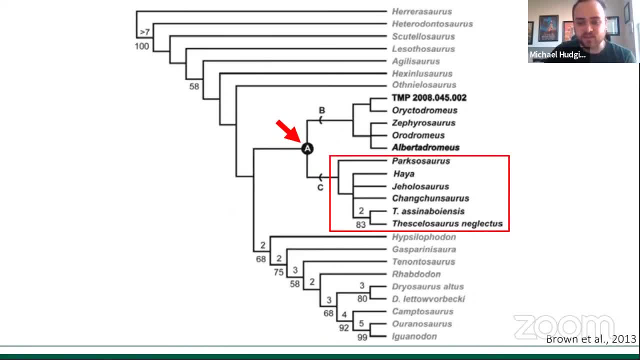 Thessalosauriens, which include Thessalosaurus, Chenchantotum and Jeholosaurus, as you see here, As well as oradromiae. Oradromiae includes oradromeus, eraseritodromeus and albertadromeus and their kin. 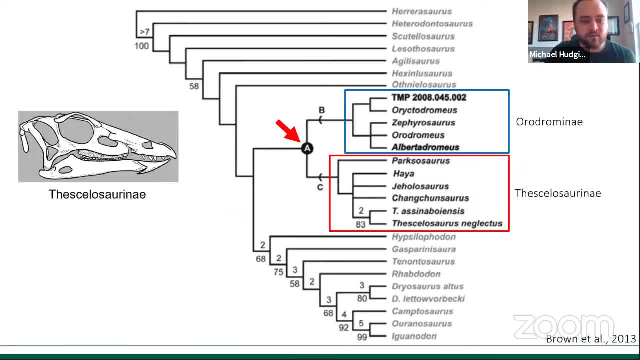 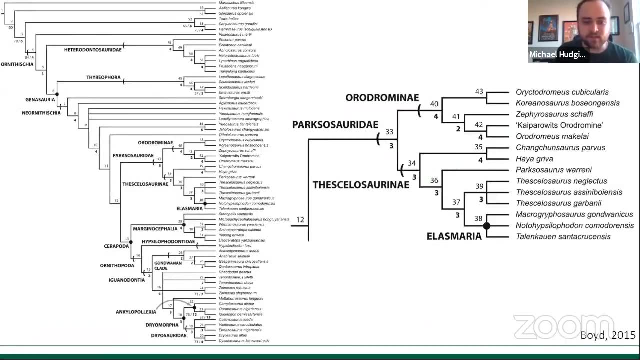 Thessalosaurinae and oradroma Theslosauriens. they have a fairly elongated snout, as you see by this thesetheslosaurus sketch- a very short snout. as you see by this orodromius sketch. Further on Boyd 2015 did a much larger. 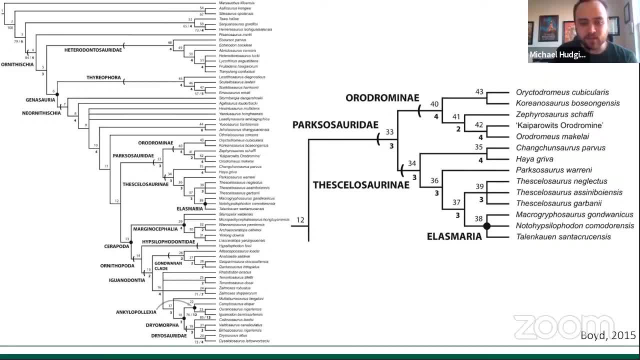 phylogenetic analysis, trying to parse together the evolutionary relationships of these basal ornithischians, As he recovered the thesosauridae, which he called Parxasauridae, which recovered thesosaurus and orodromius and rictodromius within this group, but as well as thesosaurines. 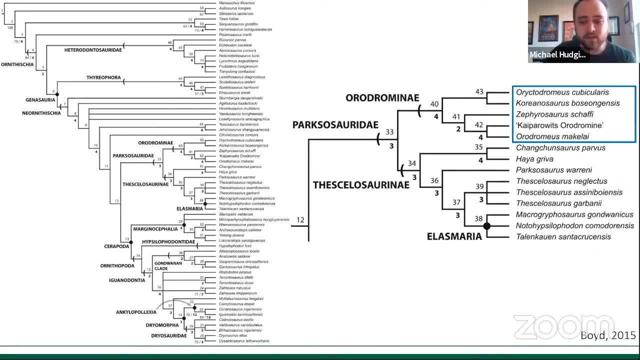 and orodromines. Orodromines are in blue with orodromius and Zephyrosaurus in their kin and thesosaurines with thesosaurus, chingchungsaurus and hya and Parxasaurus within. 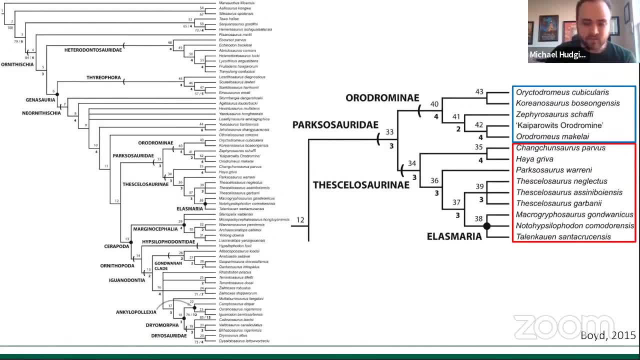 that grouping. So we have a late Cretaceous clade of basal ornithischians living alongside these larger ceratopsians and derived hadrosaurids during the late Cretaceous. even though they are basal And the relationship with subthessal sordids amongst Ornithischia and Taxa, they are sister to seropodins. 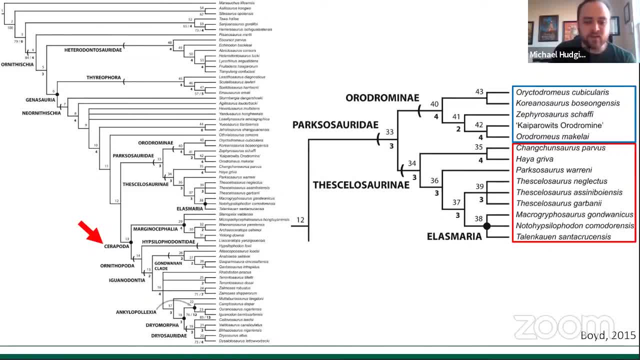 which includes marginal cephalians and ornithopods. So they're not within ornithopods, apparently, but there has been some more phylogenetic analysis that needs to be done to fully resolve this, But at this point in time they appear to be sister to seropodins. 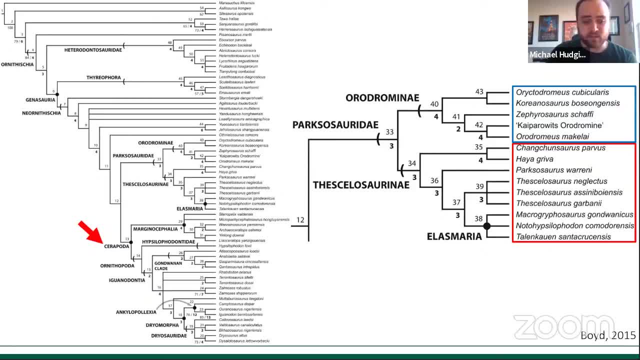 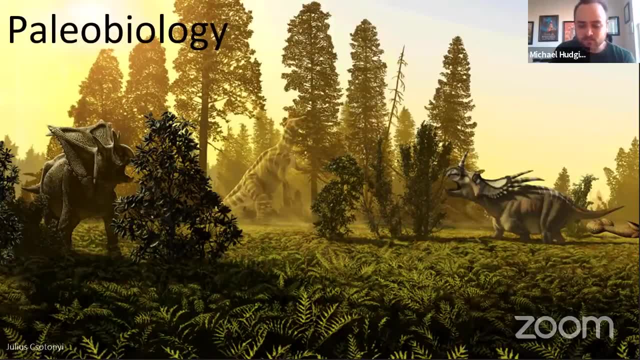 which includes marginal cephalians and ornithopods. So I'm going to talk about the paleobiology of thessal sords in general, And this is a reconstruction of the dinosaur part formation with all the large mega herbivores such as Strigosaurus, Casasaurus and Lambiosaurus. But I've noticed in this: 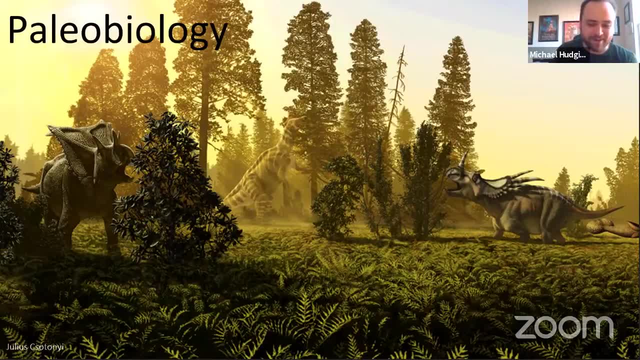 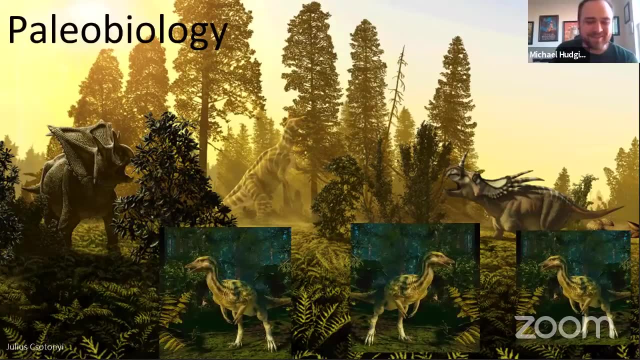 picture there wasn't a lot of. there wasn't any small-bodied ornithischia, basal ornithischia and Taxa, So I put it on myself to include these Small-bodied ornithischia and Taxa to complete the picture of the ecosystem during the campaign. 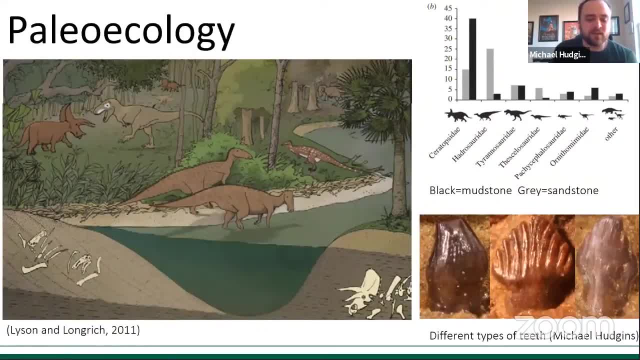 of the Cretaceous. So there was a study done by Lawson and Longridge in 2011 that tried to figure out what the preferred environments of these late Cretaceous dinosaurian Taxa. So he was looking. this group looked at the Hell Creek. 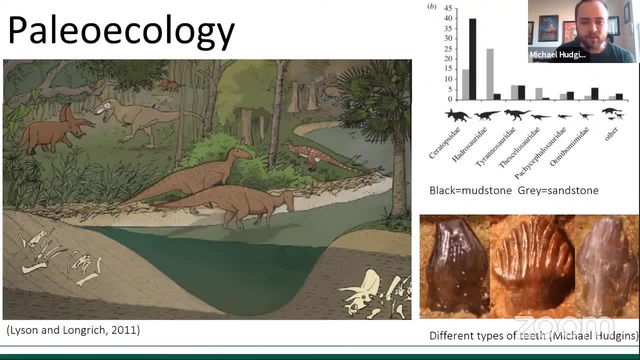 Formation and seeing which fossils are more abundant in certain rock types. So let me pull out my laser pointer. So in this graph here in the Y axis, we have the abundance of fossils and the gray and the dark boxes are representative of the type of rock. So the black box is a mudstone. 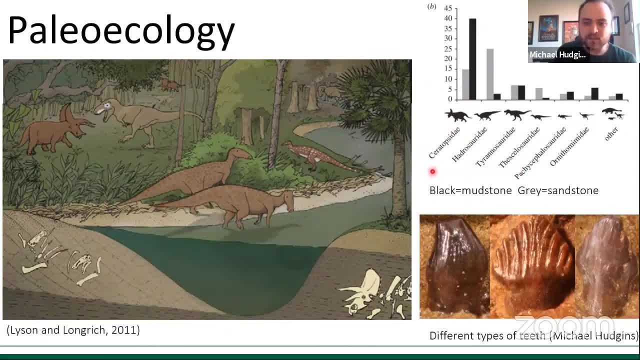 and the gray box represents a sandstone. As you see here, Ceratopsids are more found or collected more commonly in mudstone deposits as opposed to sandstone deposits, While, as Hadrosaurs are, much more are collected in more sandstone types of. 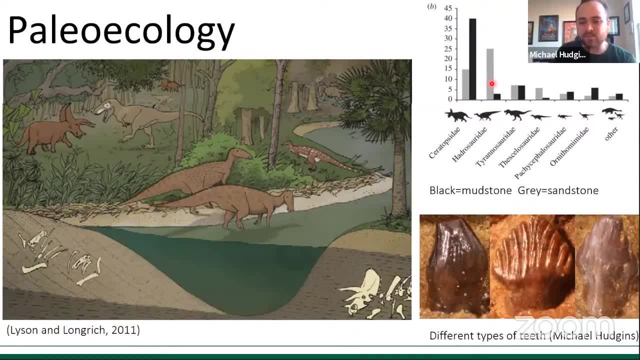 deposits they are more in mudstone types. A mudstone dichotomy is interpreted as the the abundances are interpreted as like the habitat preference. So the black boxes, for I mean so ceratopsis, are commonly found in mudstone deposits. 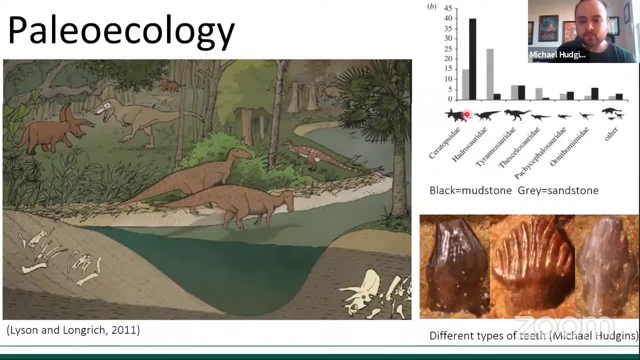 and this has been interpreted as them preferring floodplains, a type of floodplain environment, while hadrosaurs are preferred to prefer channel stone deposits and probably live close to the river's edges. And Tyrannosaurus, as you see here, is found in equally both and this. 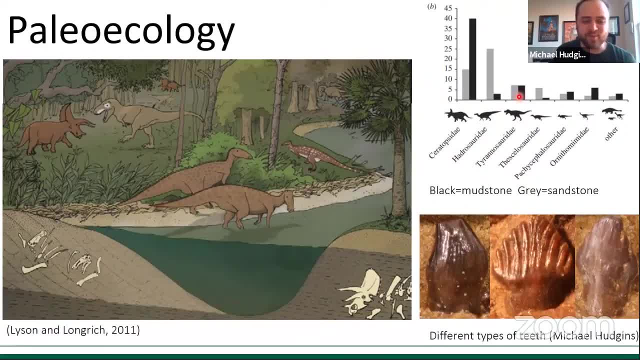 makes a little bit of sense because both their food items are living in both type of environments, so they probably don't have a preference of where they would live because they're both. they're following the food, As you see, with Thessalosaurus. Thessalosaurus is found predominantly. 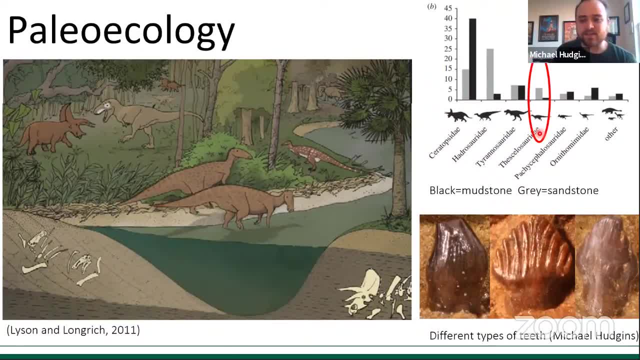 in sandstone deposits as opposed to mudstone deposits, and it's been interpreted that Thessalosaurus probably enjoyed sunny channel-side riverside environments, where they frequent the rivers and eat the vegetation along the riverbed. However, the study is still fairly. 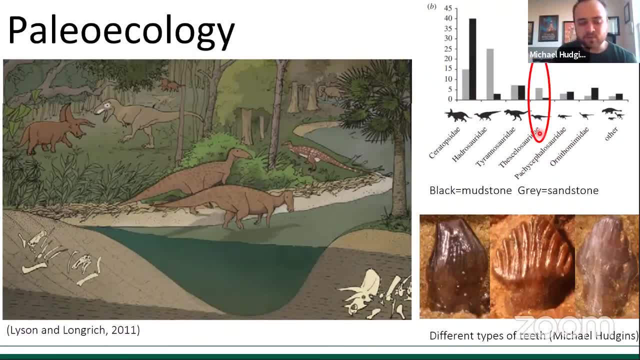 contentious about the preferred environment that these animals lived in and more studies need to be done to elucidate the ecosystem and the- I'm assuming- the environment preference for these taxidermies. So the teeth of Thessalosaurus are, fairly are, heterodont, which means they have different types. 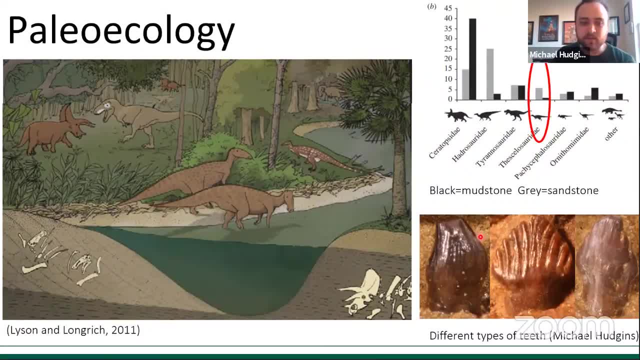 of teeth within their jawline, as opposed to, like Edmontosaurus and Triceratops, where it seems that they have pretty consistent dentition throughout their tooth row, And this has been interpreted that they have a wider range of diet. They probably ate a large selection of plants. 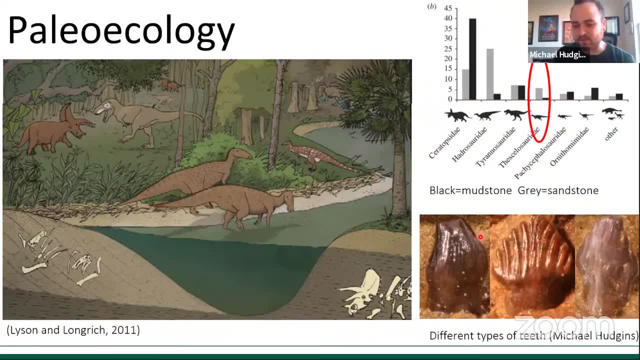 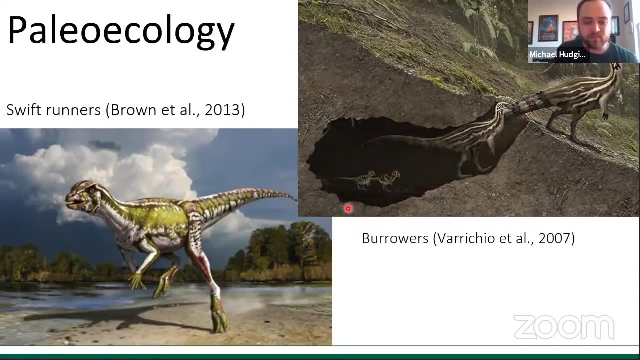 and I would not doubt that they supplement their diet for for protein, such as small lizards or or bugs as well, because of their heterodontin tition. So Thessalosaurus has also been interpreted as swift runners, based on the ratios between the 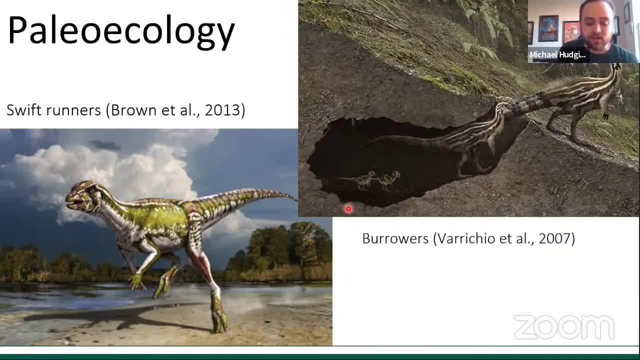 femur and the tibia. The femur is your upper limb hind limb bone and the tibia is your shin bone, And they also have been interpreted as burrowers. Back in 2007,, there was a a fossil discovery of a Thessaaura called Eryctodromeus that was recovered in a burrow-like 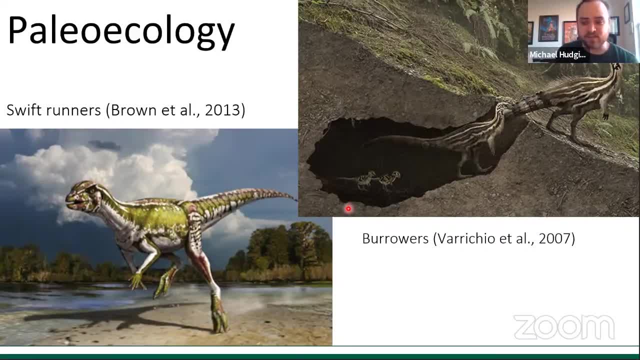 den, And this has been interpreted that these guys were, or Thessalaurs in general, were probably burrowers living in the den and probably having some form form of parental care based on the fossils that were found within that burrow, as there were adults present. 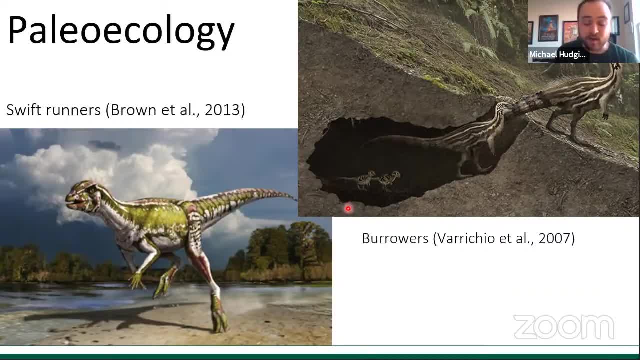 within the burrow, as well as juveniles, And also Eryctodromeus, probably would have been a swift runner because they wouldn't have eaten them. swift runner based on the femur to tibiae ratios, So Thessalaurs might have been swift runners. 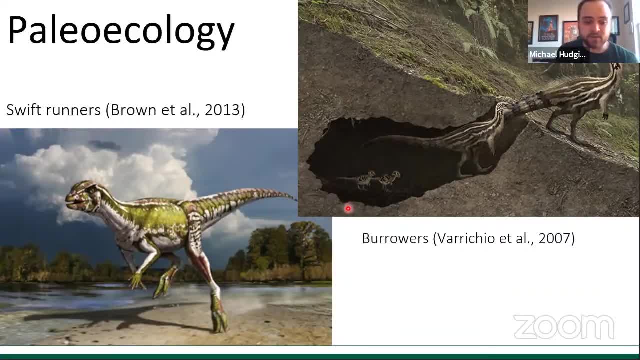 and probably denned to avoid predators as well as swiftly running away from them as well. So they have a pretty interesting paleoecology And we haven't seen burrowing. This is the first instance of a dinosaur being able to burrow And I don't think we have discovered another. 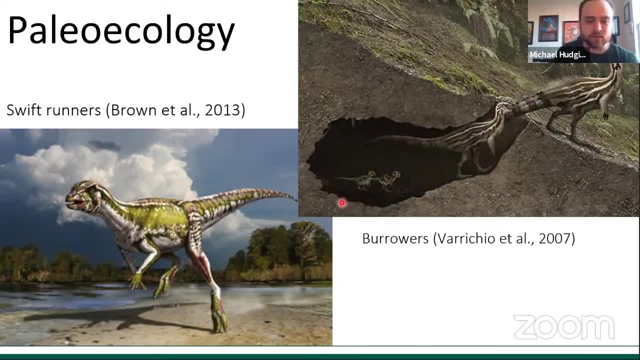 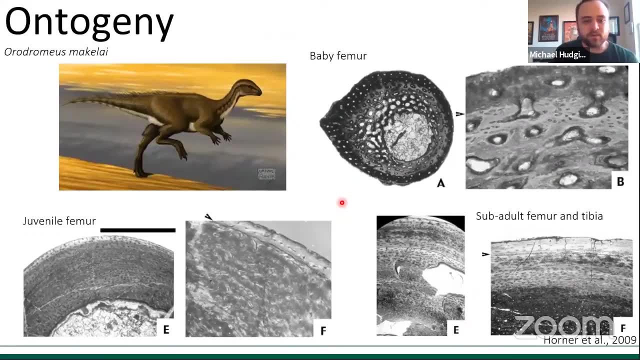 dinosaur or outside of Thessalaurs that would be able to burrow. So the growth stages or the growth of these animals of Thessalaurs is fairly unknown, And this is called ontogeny, And so not a lot of work of understanding their growth has been conducted. 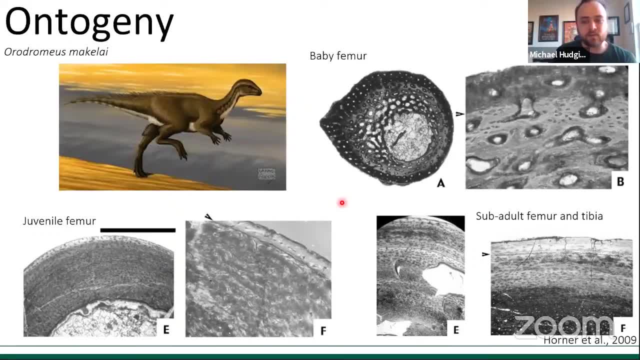 Only a few examples, such as Orodromius, as well as Eryctodromius and Thessalaurs And some of Jeholasaurs, But there's only a couple studies looking at bone histology of Thessalaurs, And bone histology is taking bones and slicing them and taking those really. 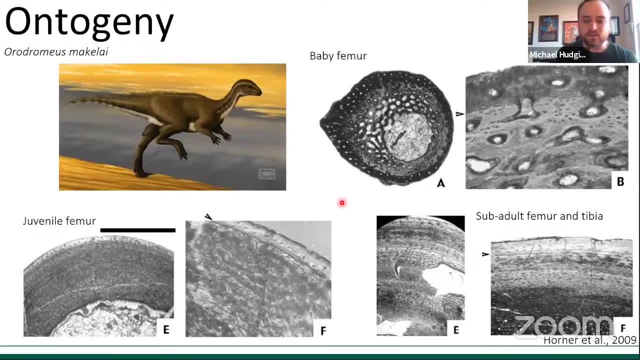 thin sliced section, putting them under a microscope and understanding their growth rates and what kind of features they have within their cross section. And so here we have an example of Orodromius, of a baby femur, a juvenile femur and a sub-adult femur or tibia. 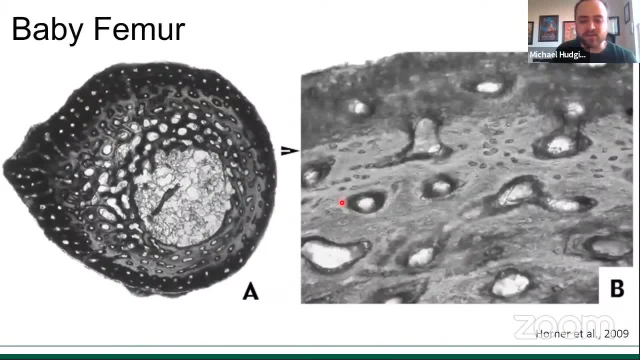 So with the baby femur it's fairly vascularized, with a lot of blood vessels, And this is signifying that the animal was growing fairly rapidly and is still a very young, young animal. There are no lags or lines of arrested growth, which is basically like the tree rings of animals. 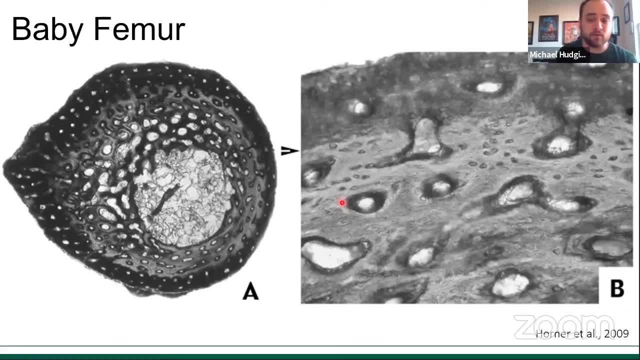 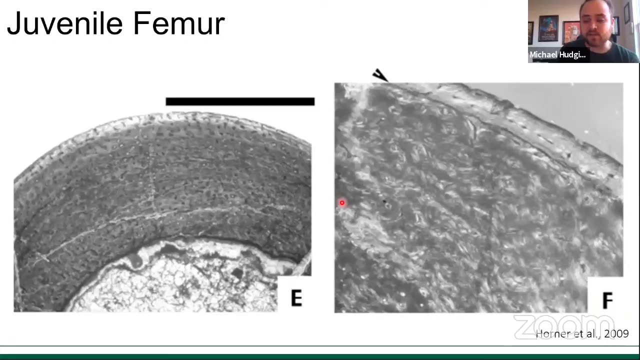 This signifies how old they are And there are no lags within this baby femur, So it's suggesting that this animal was still growing and less than a year old. The juvenile femur has less vascularization towards the edge of the bone, as you see here more. 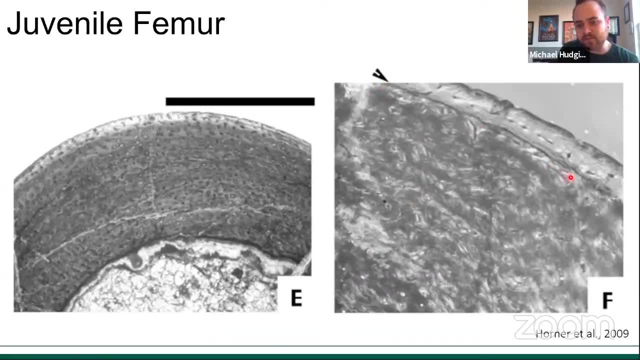 vascularized towards the center And they have one line of arrested growth here And this signifies that the animal is growing and is older than the baby, is about one years old, But it's slowing down in growth because there's less vascularization present on the animal, suggesting the animal is 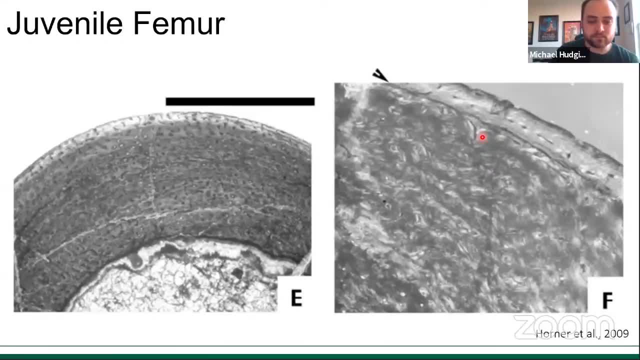 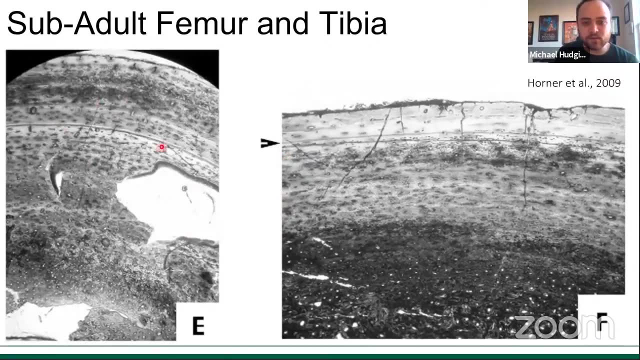 older, but not quite at adult age yet, And the adult femur, sub-adult femur and tibia has more lines of arrested growth, as you see here, and the vascularization from the inner bone to the outer bone decreases substantially, with the outer bone having less vascularization compared to the inner bone. 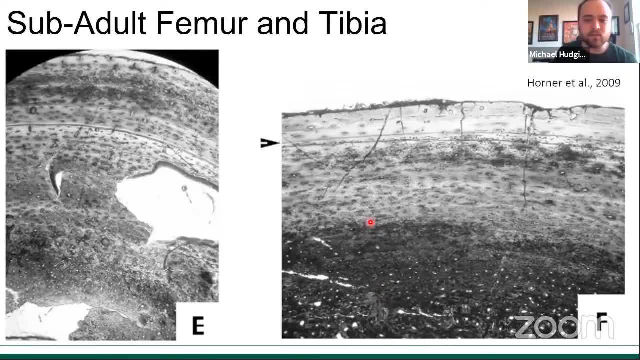 And the lags for the subadult femur and tibia for orodromius is roughly between two to three years old, depending on which element you're looking at and which individual you're looking at. So the maximum age for these animals might be around three or four years old potentially. 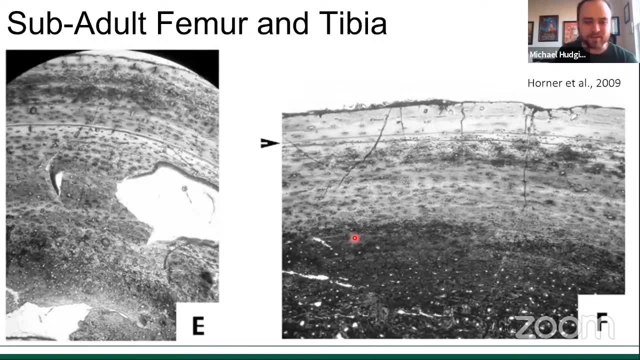 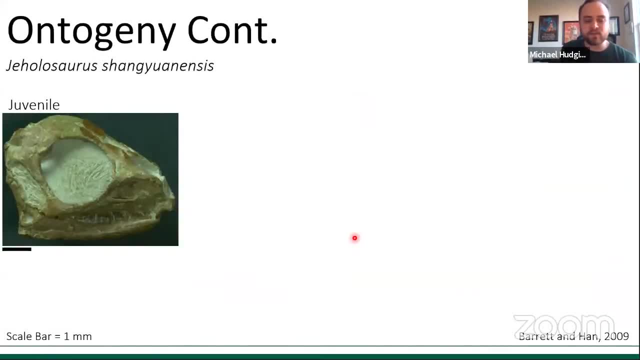 But they lived pretty quickly compared to other dinosaurian taxa. So here's a continuation of ontogeny And this is geholosaurus. Like I said, might be outside of Thessalosauridae, depending on which phylogenetic analysis that 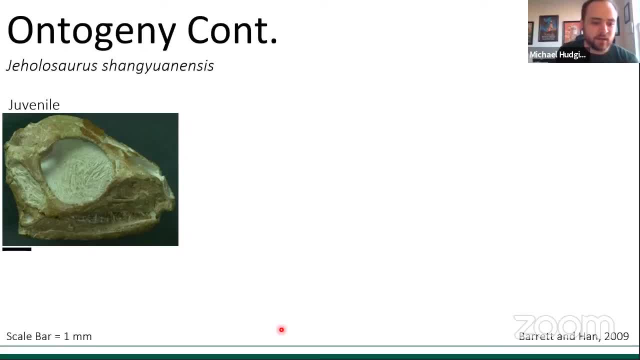 you are looking at, And so we have a juvenile geholosaurus right here with large eyes And, if you notice, it has a very short snout, And when we look at more, when we look at juvenile specimens, the snout gets larger. 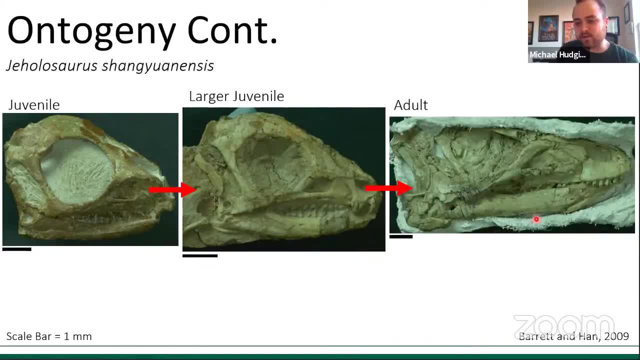 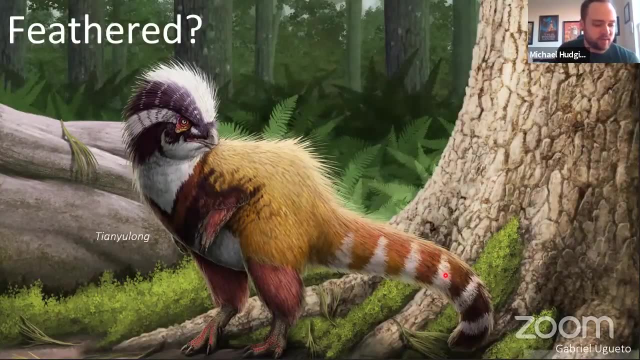 And then when you look at the fully adult specimens, the snout gets even more larger. As you see, you have a progression from shorter snout to larger snout as the animal gets older, which is actually quite interesting. So an interesting question about the paleobiology of Thessalosaurus is: what did they look like in real life? 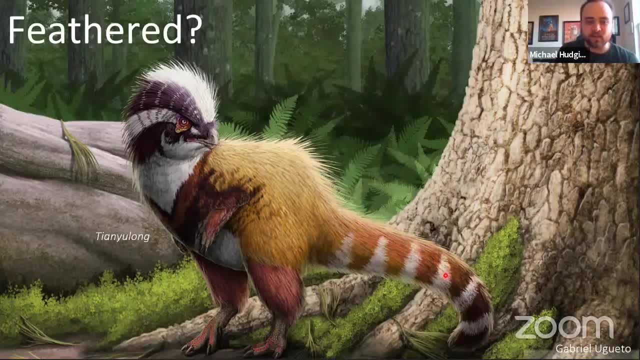 What sort of integument do they have? Were they feathered or were they scaly? And here's an example of not a Thessalosaur, but an animal called in the group Heterodontosaur, which is a. this is a Jurassic animal called Tian Yulong. 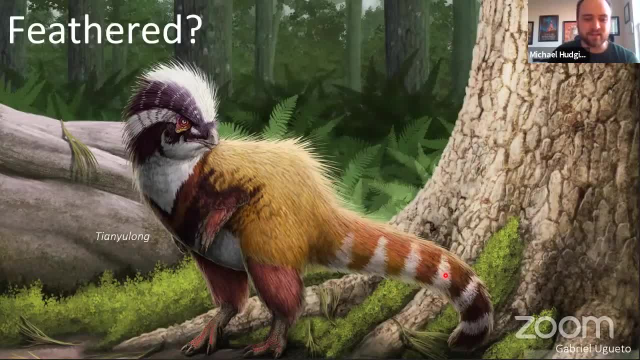 And it's a Heterodontosaur, like I said, and it's been interpreted as being fully feathered, And it questions whether or not Thessalosaurs or these basal ornithischian taxa, were fully feathered as well or were scaly. 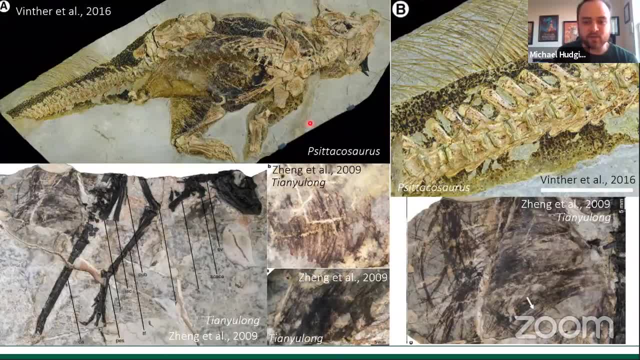 So we have a couple of examples. We have Psittacosaurus, which is a basal ceratopsid, and Tian Yulong, which is the Heterodontosaur we saw earlier And, as you see over here, that Psittacosaurus, on the tail has these bristle-like filaments, like structures. 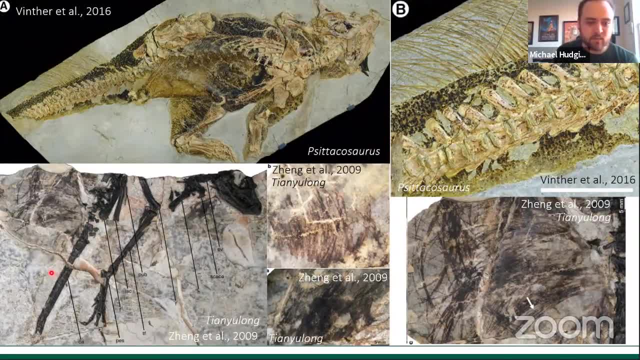 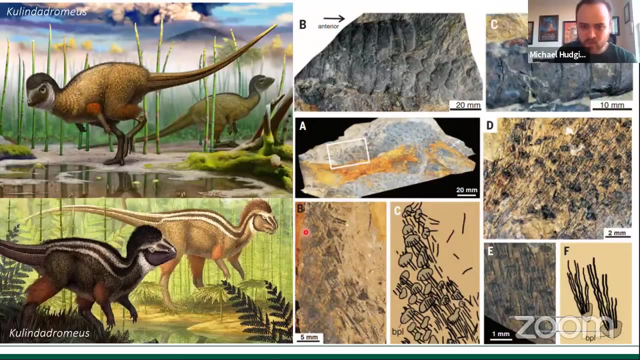 Whether they're feathers is up for debate still. And the same thing with Tian Yulong, which has these bristle-like feathers or integument on the back of the animal. With this, there has been a discovery called Culana didromyus, which also has feathered integument, or feather-like integument on the body of the animal. 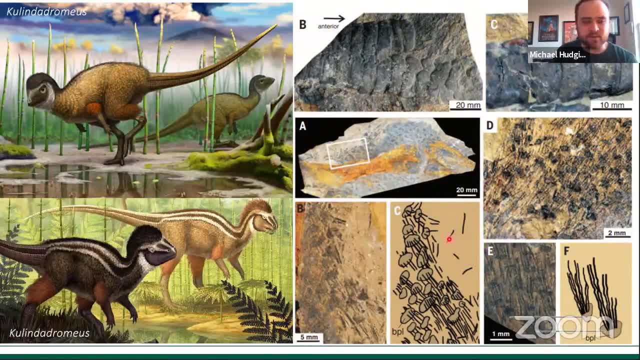 These feather-like integuments don't look like the feathers that we see on birds. They're not panaceous, But they have like these filament-like tufts along the body of the animal. But what also is really cool is that the tail has this, and the tail and the hind legs. 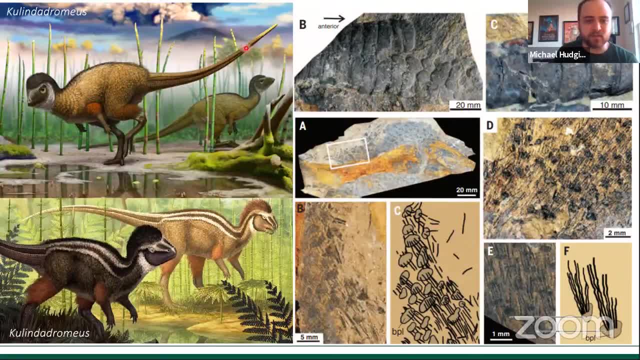 The tail and the hind limb- the bottom of the hind limb- have these keratinous-like scales along the tail and the hind limb, at the bottom of the hind limb, as you see here, Which is kind of fairly interesting given that Thessalosaurids are fairly closely related to these guys, and they might actually look like this. 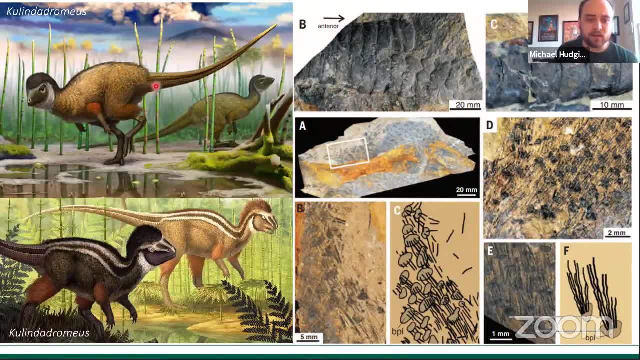 But this animal would have fully tufts on its body, a tail that was fully keratinous with scales, and the bottom part of the foot would be keratinous with scales, just like a chicken. But this animal would have been probably the size of a dog and it looks- the reconstruction looks- fairly cute. 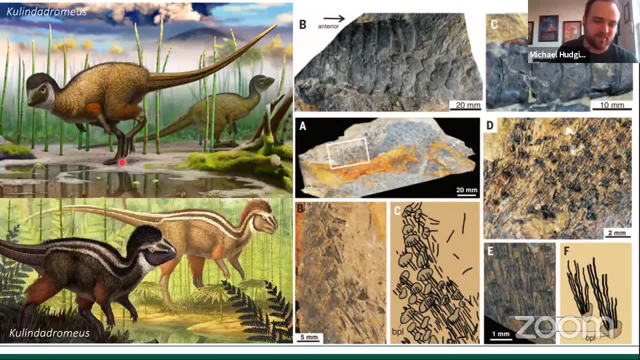 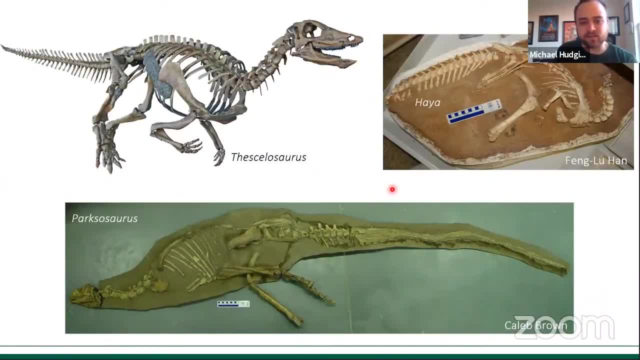 I would not imagine this animal was still around today, that this would be a pet. So this leads to the question whether or not these Thessalosaurid taxa from the late Cretaceous period were also, and fully were, have some form of integument along its body. 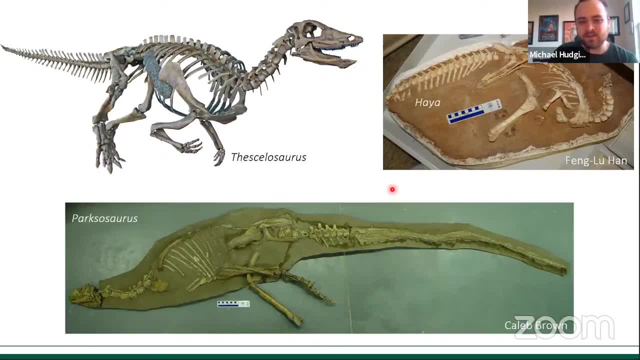 And we don't have any of that soft tissue, integument or skin presence. So we really don't know what these guys look like in real life, And so you can reconstruct them either way, potentially either having some form of integument on their body or fully scaled. 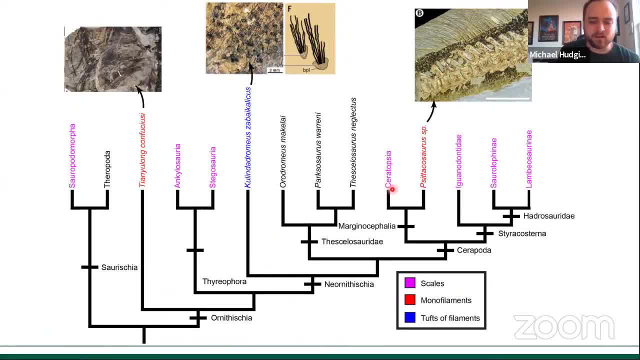 But we can also look at the phylogeny of these animals, such as Cuolana, didromus, Tian yulong and Psittacosaurus, and where these integuments fall on the family tree. So we can get a pretty good estimation of whether or not these 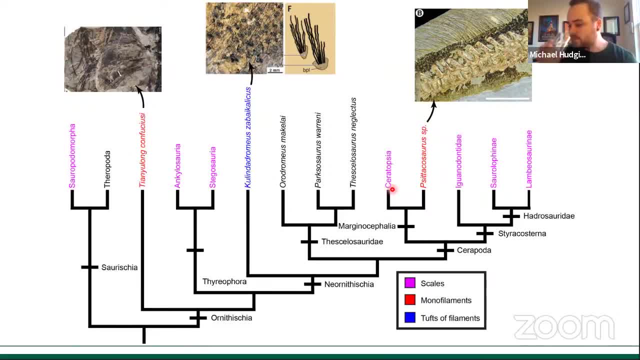 Thessalosaurid taxa were fully feathered or not? So, with Psittacosaurus being a marginal cephalian really closely related to Ceratopsia, and Tian yulong is fairly basal on the Ornithischian tree and the Cuolana didromus is fairly closely related to Thessalosaurids. 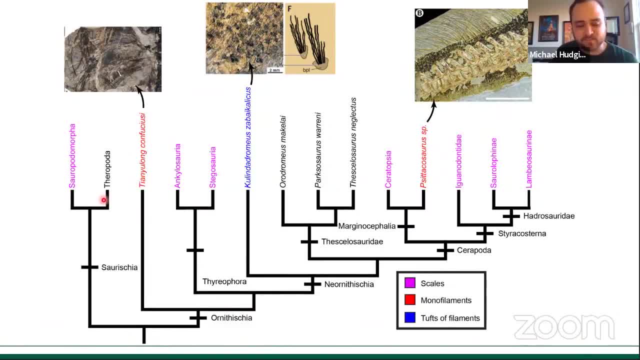 I'm sorry, I should have backed up a little bit. So this is a color-coded phylogeny And Scales are in pink or purple. Monofilaments which were present in Tian yulong and Psittacosaurus were in red. 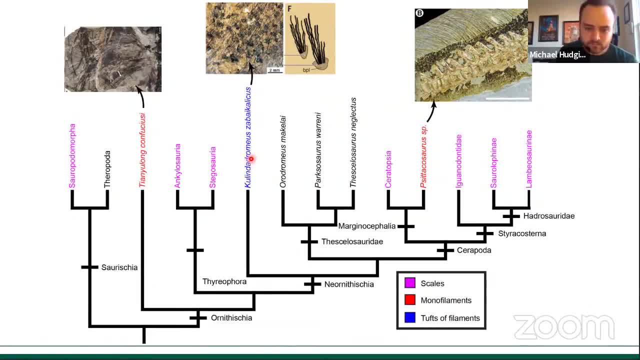 And the tufts of filaments were in blue for Cuolana didromus. As you see here that Tian yulong is fairly basal in Ornithischian standards and Psittacosaurus being closely related to Ceratopsia, late Cretaceous Ceratopsia. 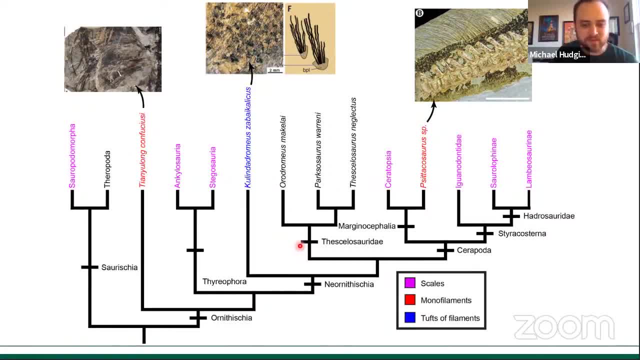 And Cuolana didromus is fairly. It's fairly basal to Thessalosaurids and Ceropodins as well, So you can interpret Thessalosaurids as having either scaly skin or some type of scale, some type of monofilament or tufts of filaments on its body. 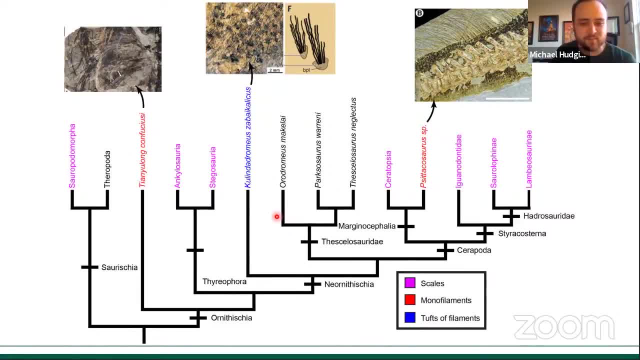 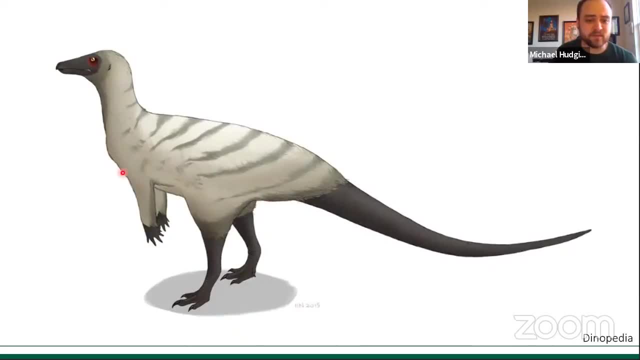 But it's really hard to say based on we don't have any of that skin preserved on the body of the animal, of these animals, excuse me, So you can interpret this as, like I said, as being feathered with a body, something similar to Cuolana didromus with the feathers. 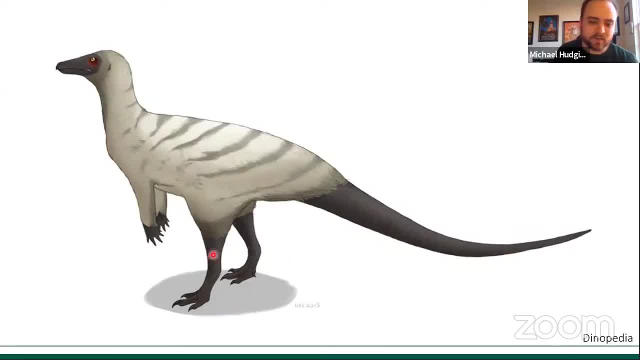 The tail being keratinous with scales and the bottom of the feet being keratinous with scales as well. Or you can interpret these guys, these Thessalosaurid taxa, as being fully scaly as well. Until we get skin preservation of Thessalosaurids within the fossil record, it's really up in the air what these guys look like. 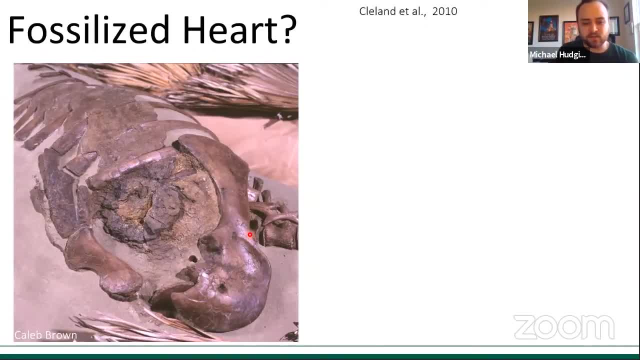 So in 2000, there was a paper describing a Thessalosaurus From the Hill Creek Formation that was potentially having a heart. This specimen is called the Willow specimen and is now housed in North Carolina State Museum, And the original authors who described the specimen thought this mass in the chest cavity of this Thessalosaurus specimen was a potential fossilized heart. 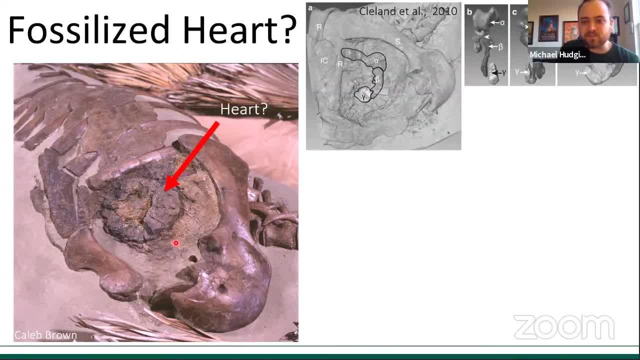 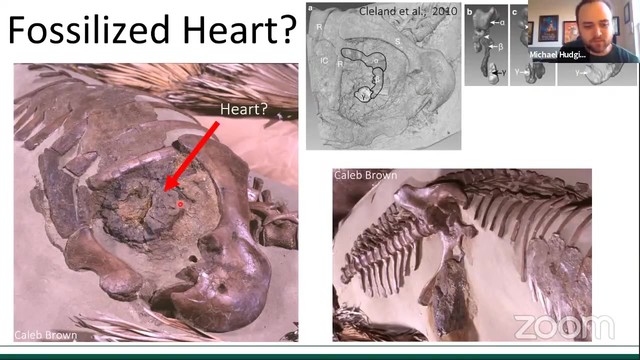 And so the scientists did some CT scans And what they thought they found Were the valves of this supposed heart in Thessalosaurus. But under close examination there was other types of this morphology around the skeleton of the animal of Thessalosaurus that were fairly similar to the composition and morphology of the supposed heart. 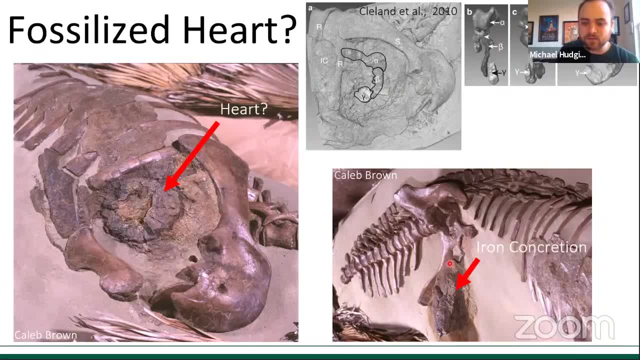 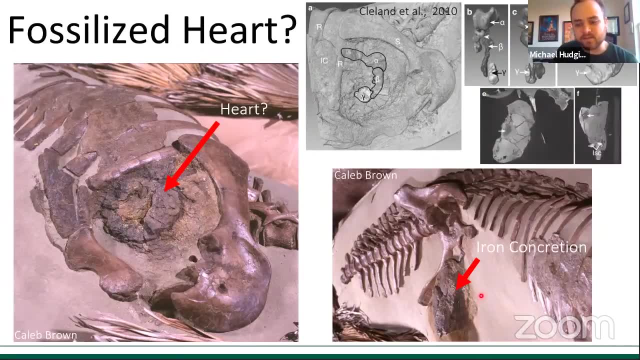 So this thing at the bottom of the hip is an iron, The hip is an iron concretion. It's just pure iron And they did a CT scan and did some composition work and it has the same morphology as the supposed heart, with the iron concretion towards the hip, and it's made of the same material. 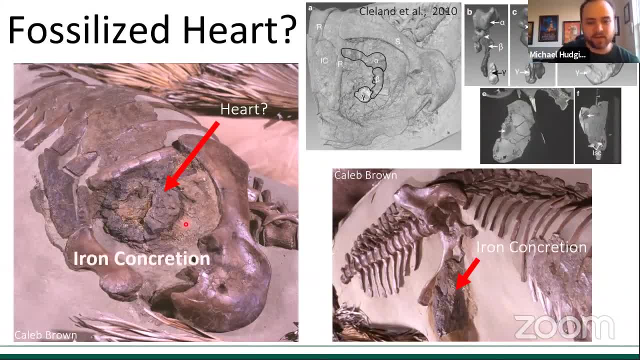 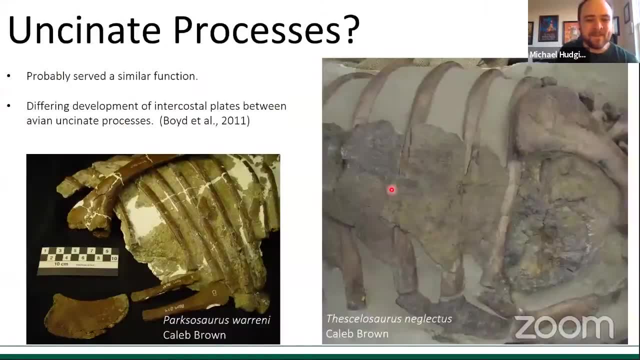 So it's very likely that this is not a heart but in actuality is an iron concretion. So dang it. So further on About their paleobiology, we have potential uncinate processes or structures that are similar in function with uncinate processes. 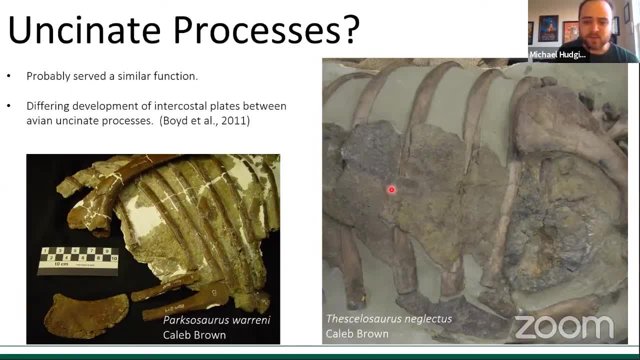 And uncinate processes are typically found in theropod dinosaurs, as well as modern day birds, that assist in the breathing and respiration of these animals, And so these intercostal plates, that which are called in Thessalosaurus, probably pose a similar function to. 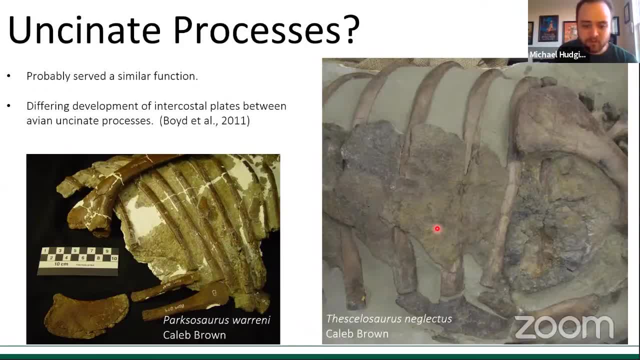 uncinate processes seen in theropods and birds. However, as you see, in Parxasaurus here those are the intercostal plates and these are the intercostal plates for Thessalosaurus. However, the development of these intercostal plates in Thessalosaurus developed differently from the uncinate processes in birds. 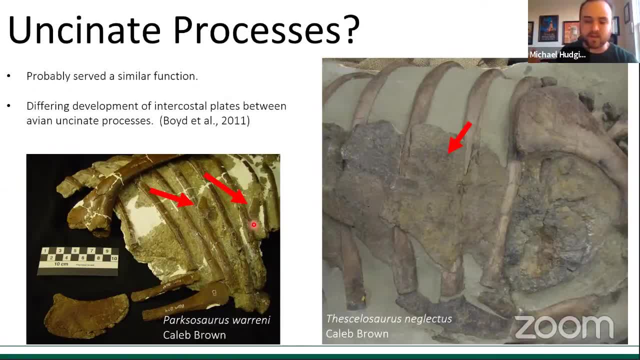 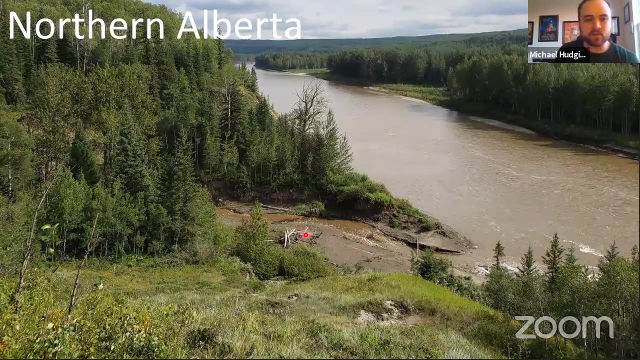 And so the uncinate processes in birds ossify from the out to the inward, and what the intercostal plates for Thessalosaurus? they ossify from inward to outward. So a completely different osteogenesis. So segwaying out of the paleobiology of Thessalosaurus. we're going to talk about my research up in northern Alberta. that's been predominantly my master's thesis. 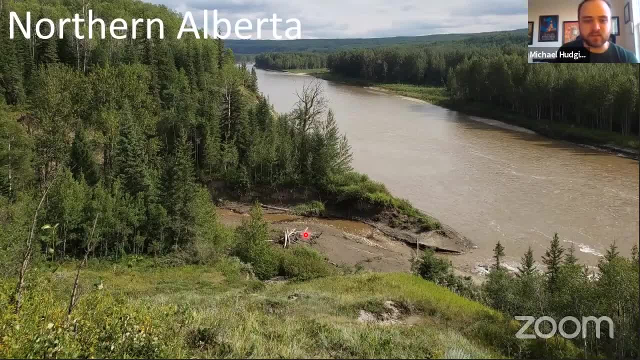 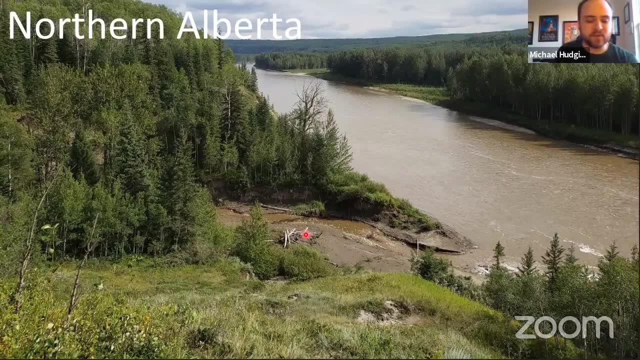 And we've been describing new Thessalosaur material from the dc bone bed uh up in uh grand prairie, uh, canada, and it's. this material is fairly important, uh, for a number of reasons, which i'll continue in a second, but this material is coming from the 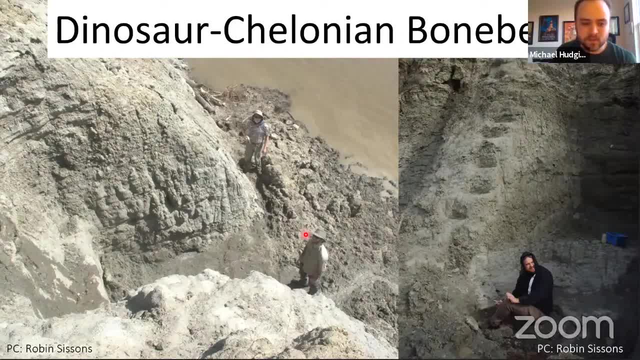 dana chelonian bone bed, or the dc bone bed, like i said, and it's a fairly small quarry uh along the wapiti river and it's a quite a terrifying climb down. i am definitely afraid of heights, but the only way to get down to the quarry level is taking these uh self-made stairs in the cliff. 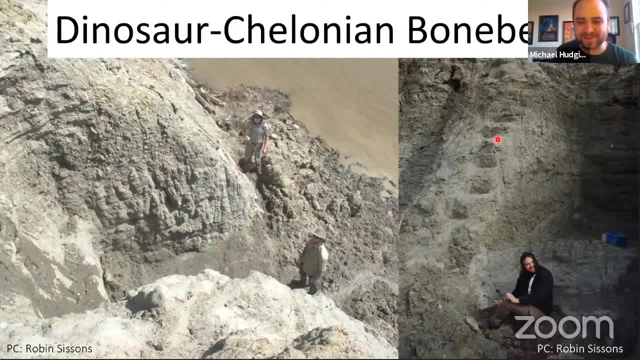 face to get down and when i was there i was shaking very, very uncomfortably- uh, going down- because me and heights are not best friends. but the quarry is pretty cool. it's very muddy and very small but it has a lot of fossil material of thessal swords coming out of this. 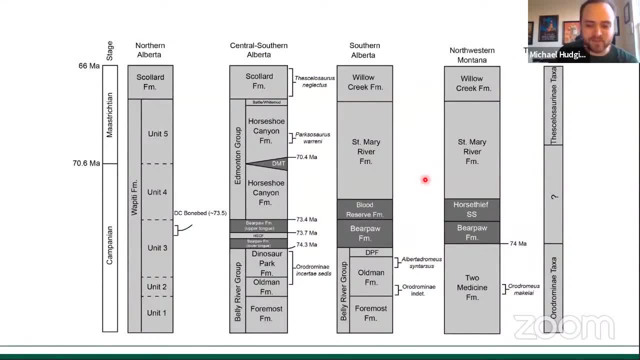 and so the importance for this fossil material is quite interesting. so here is a stratigraphic uh, stratigraphic columns of northern alberta, southern alberta, central southern alberta, northwestern montana, as well as thessal sword occurrences, and so the way to read this is: here's the time scale, right here. here's the 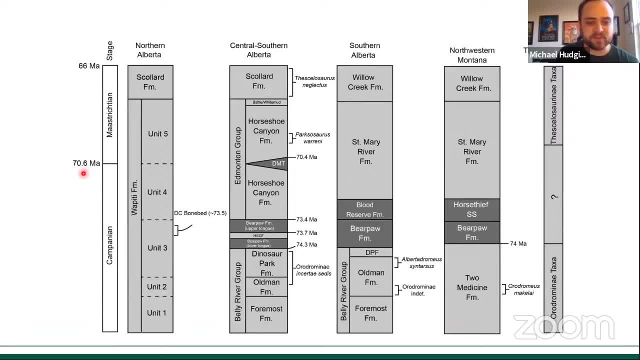 campanian, then the maastrichtian, and this is this line right here- represents 70.6 million years ago, and this is 66 million years ago, which represents the age of the end of the dinosaurs. and so anything at the bottom is older, anything at the top is younger, and all these boxes here, 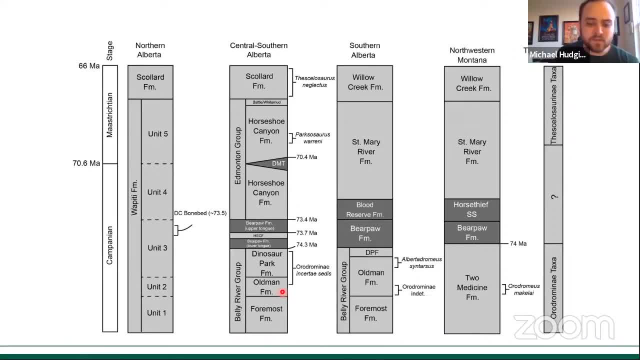 represent rock formations, and so the gray represents terrestrial environments and the dark gray represents marine environments. so in the older um belly river group of alberta, in southern alberta and in northwestern montana or dromina, taxa are only found in these old boxes, and so we can see that these boxes here are these rock. 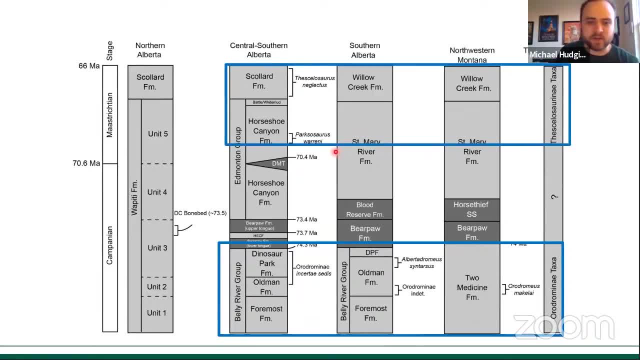 water sediments, While in younger strata, in the Horseshoe Canyon Formation and the Scholar Formation, only Thessalsaurinae taxa have been discovered so far. And so in between these two stratigraphic units, between the Horseshoe Canyon Formation and the Dinosaur Park Formation, we have 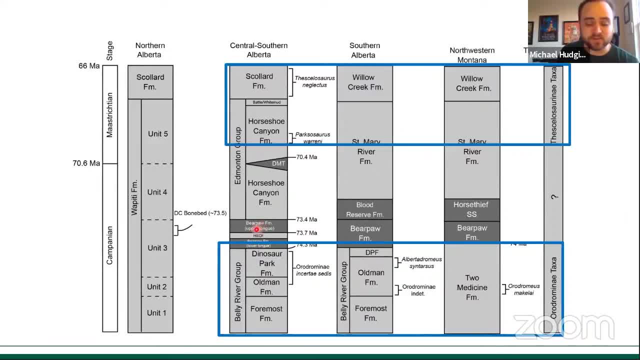 this marine interval called the Bear Paw Formation in central southern Alberta, which basically truncates the evolution between Orodrominae taxa to younger Thessalsaurinae taxa. So we don't really know if there's a turnover event or if Orodromines become Thessalsaurines. 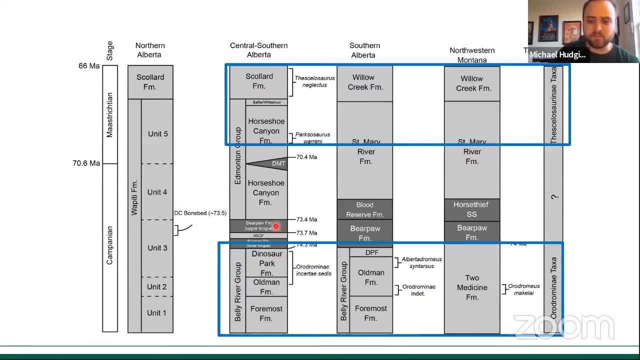 we don't really know, But the DC bone bed appears to be a terrestrial representation of the Bear Paw Formation. So the Wapiti Formation records the entire terrestrial sequence between the Campinas and the Bear Paw Formation. And so the Bear Paw Formation records the entire terrestrial 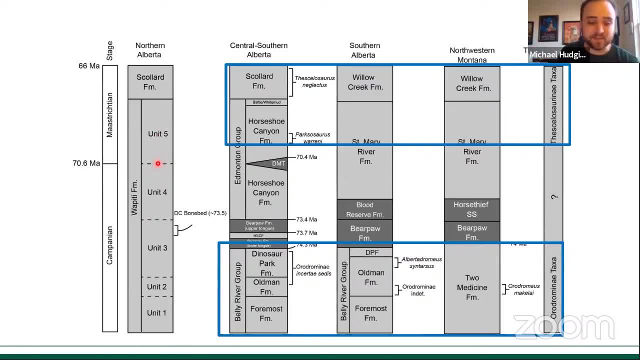 sequence between the Campinas and the Bear Paw Formation, And so the Bear Paw Formation records all the way to the Maastrichtian and thus provides insight about the evolution of Thessalsaurids during this time frame. because of the truncation of the Bear Paw Formation, obscuring the Thessalsaurid, 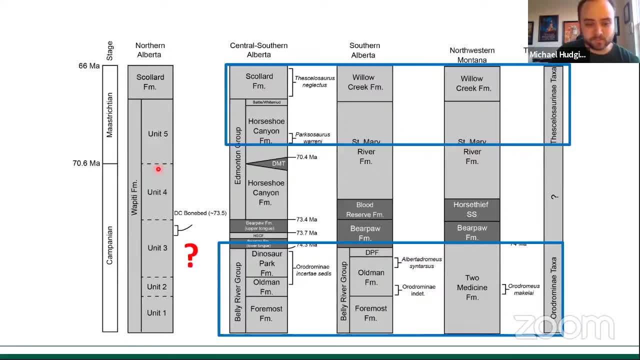 evolution during that time period in southern Alberta. So I was trying to figure out what these fossils represent, whether or not, coming from the DC bone bed, represent a Thessalsaurid, and hopefully elucidate the evolution of these of this group during the late Cretaceous of North. 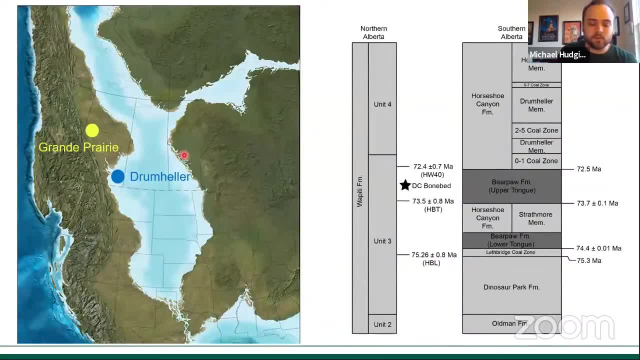 America. So here is a reconstruction of the paleogeography during the Bear Paw Formation times, And Drumheller at that time frame would be underwater but Grand Prairie would be terrestrial and we can get fossils from that time period to understand what is going on during that time period. 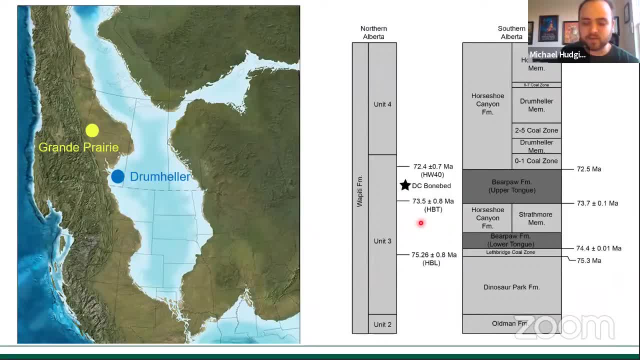 And so the DC bone bed is in between two dated rock units around 73 million years ago, or it's between 73 million years ago and 72 million years ago, which coincides roughly with the Bear Paw Formation. So the DC bone bed represents that missing time interval between older Orodromine. 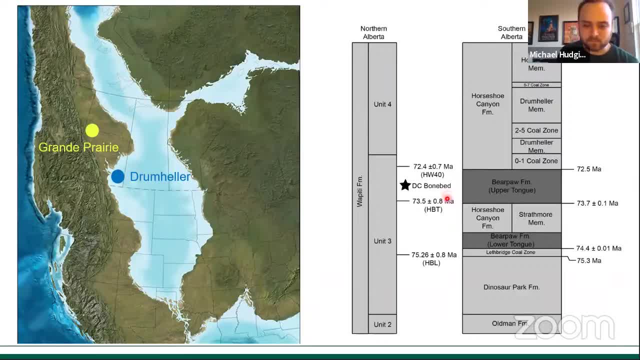 taxa and younger Thessalsaurid taxa. So for understanding this, I'm going to go ahead and do a little bit of a quick analysis here. So understanding what this material is is pretty crucial into understanding what's going on in North America and these basal ornithischine groups. 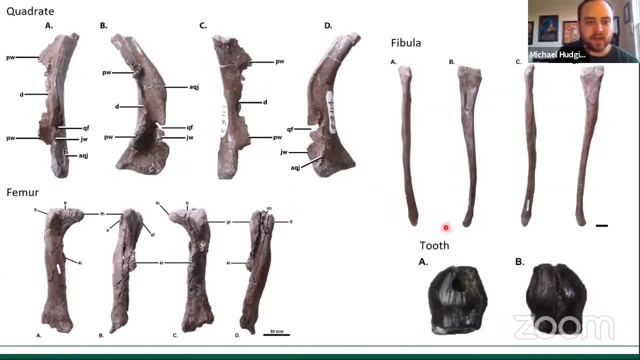 during the Late Cretaceous period, And so we have a few fossils here of the DC bone bed Thessalsaurid. We have the quadrate which is part of the skull of the animal, The femur, which is the upper bone. 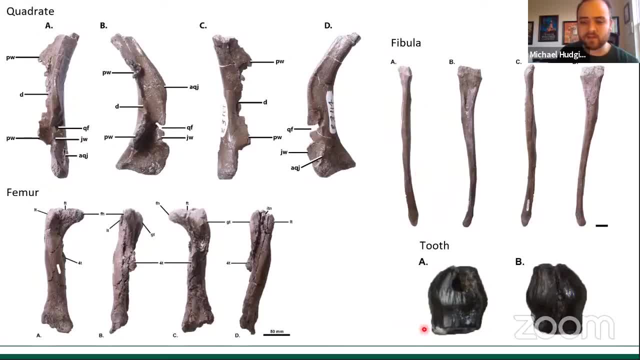 upper hind limb bone of the animal And we have the fibula and tooth. The fibula is the tip of the bone, is part of the shin bone. The shin bone makes up two bones, the tibia and the fibula, So the 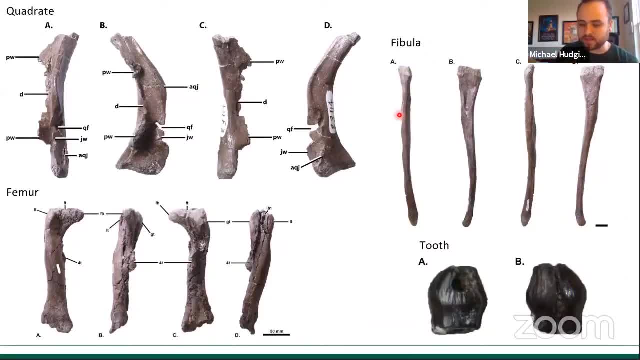 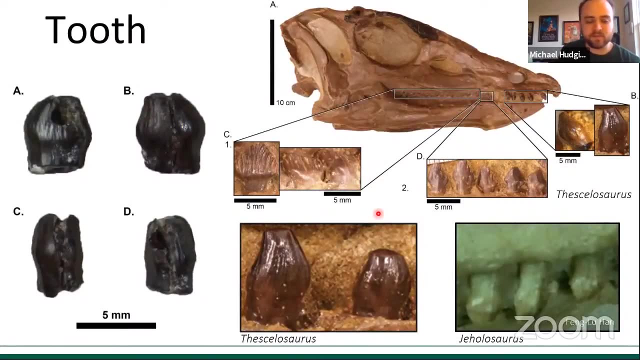 next time you eat a chicken bone, that little splint of bone that you take off from the larger bone of the chicken bone, that is the fibula. So this is the fibula of this potential Thessalsaurid. So the tooth from this quarry is fairly similar to Thessasaurus or Thessalsaurid teeth. 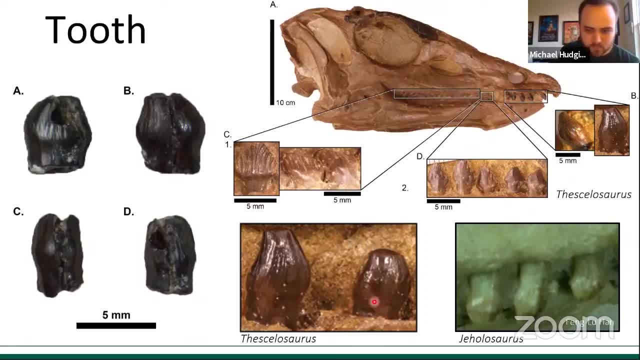 The tooth is fairly bulbous, just like Thessasaurus neglectus, as well as Jeholasaurus, and also as well as Changchangsaurus and Haia, But what's unique about this is that it has these vertical ridges running along the tooth itself, fairly similar to Thessasaurus neglectus. 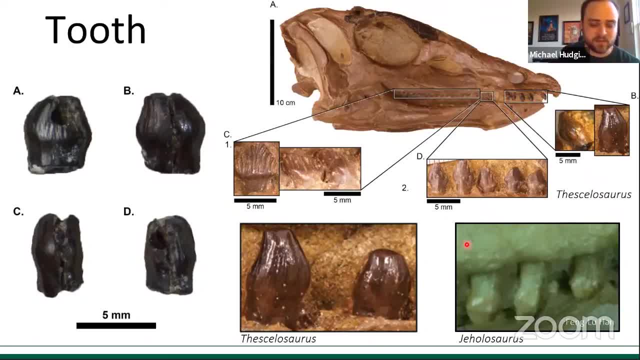 but not really with Jeholasaurus or any other Thessasaurid taxa, especially not just Jeholasaurus or Haia, And so this tooth is fairly similar morphologically, and the features present on this tooth are fairly similar to Thessasaurus neglectus, And so it appears that 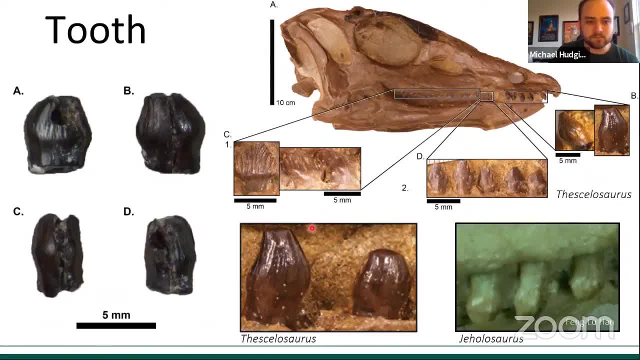 it would be a Thessasaurid, based on just this tooth right here- And I forget to mention that this tooth was found- is most likely representing the front upper teeth of a Thessasaurid, not the back teeth, But a front premaxillary tooth of this animal. 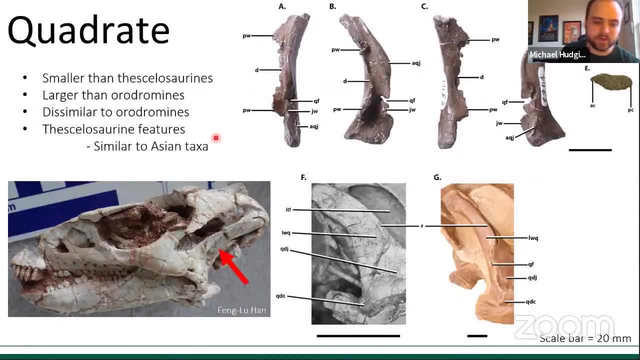 So this element right here is called the quadrate, And the quadrate is found along the skull, the back of the skull, and acts as like a hinge, acts as a hinge joint for the lower jaw. The quadrate from the DC bone bed is quite morphologically similar to Thessalsaurines. 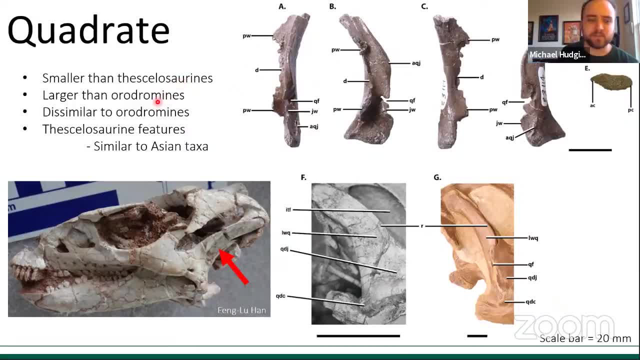 but it is smaller than Thessasaurus. It is smaller than Thessasaurian quadrates but it is, however, larger than Orodromine quadrates. Morphologically, the DC bone bed is very dissimilar from Orodromine quadrate. They have a fairly 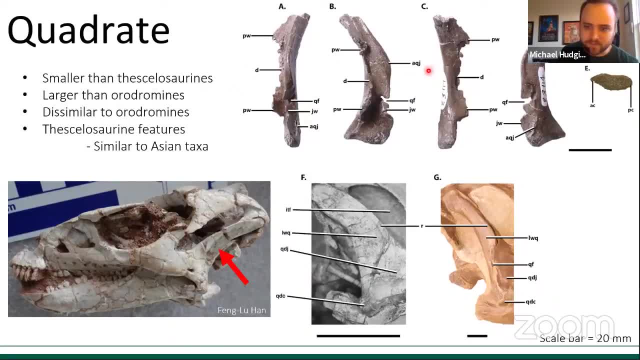 different morphological features that are not that don't really look like the DC bone bed, But the DC bone bed quadrate looks very, very similar to the quadrate of Thessasaurines, such as Thessasaurus neglectus and Changchunxaurus, as well as Haia. 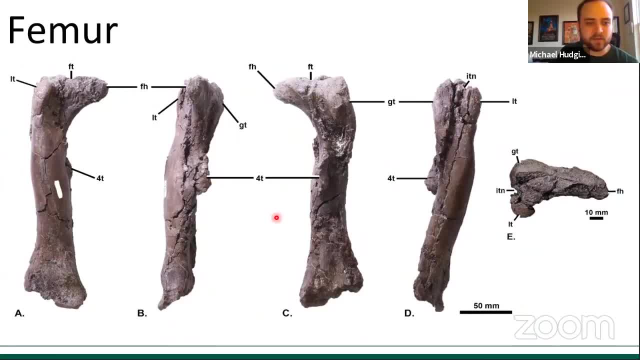 So the femur is very similar to Orodromine quadrate And the femur is not a particular feature that is known to be very different from Orodromine quadrate. The femur is fairly interesting in the DC bone bed. It's got the features of a dinosaur. 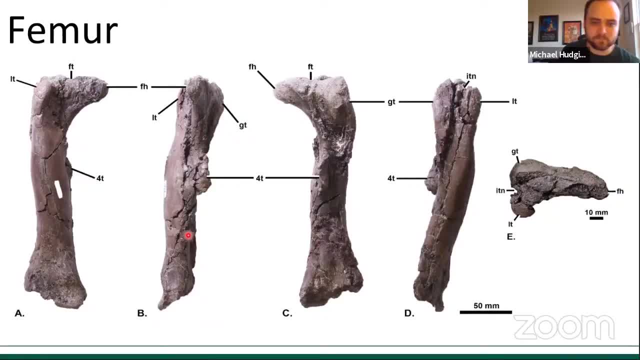 the fourth trochanter- And it's pretty diagnostic of a dinosaur. The fourth trochanter is basically the diagnostic feature, like I said, of Dinosauria, but also acts as a main retraction for the femur when in locomotion. 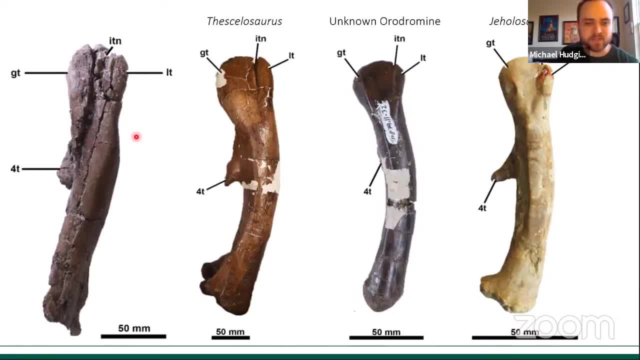 femur with all other Thessalosaurid taxa as well as other Late Cretaceous Dinosaurian taxa. but the DC bone bed is very, very similar to other Thessalosaurid femurs. They're bowed. they're all bowed as well as the fourth. trochanter is rather pendant shape. The fourth 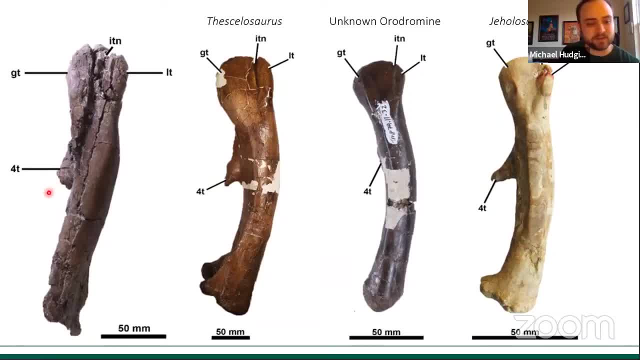 trochanter on the DC bone bed is damaged at the distal end, but it would have extended further down based on that damage. So it had a fairly pendant. fourth trochanter: just like other Thessalosaurid taxa, They also have this cleft that separates the lesser trochanter. 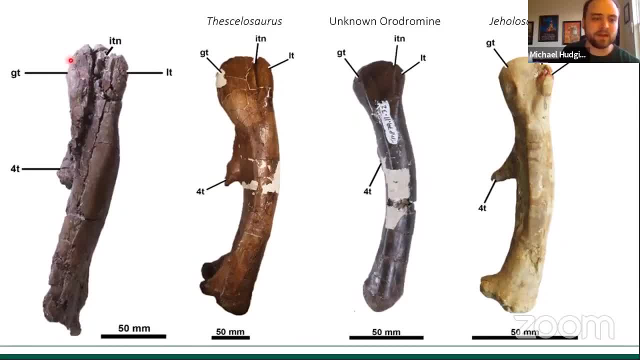 which is a muscle attachment site for the animal in life, as well as the greater trochanter, which is also another muscle attachment site that is similar to other Thessalosaurs. They have that cleft that separates them out, But what's interesting is that the femur is fairly 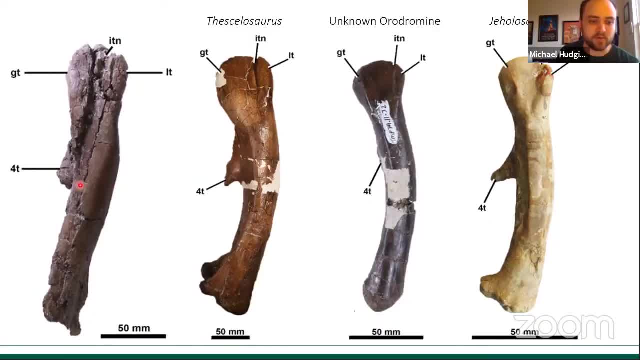 robust compared to other Thessalosaurs, but the femur is not as robust as the Thessalosaurids, So it's not as robust as the Thessalosaurids, but it's not as robust as the Thessalosaurids. 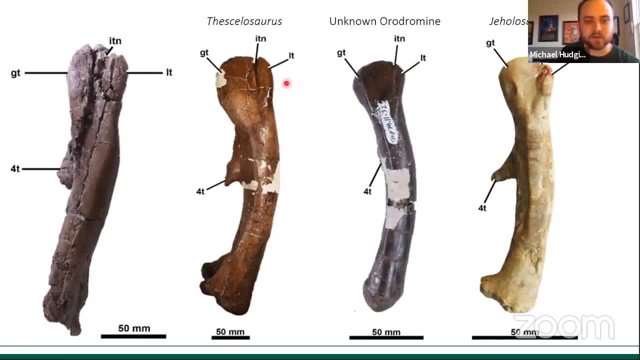 Both in width and also the lesser. trochanter is fairly large compared to much larger Thessalosaurid animals, And so that made me question: is there a way to quantify how robust this femur is compared to other Thessalosaurids, Thessalosaurid femur femora? And so I did a simple. 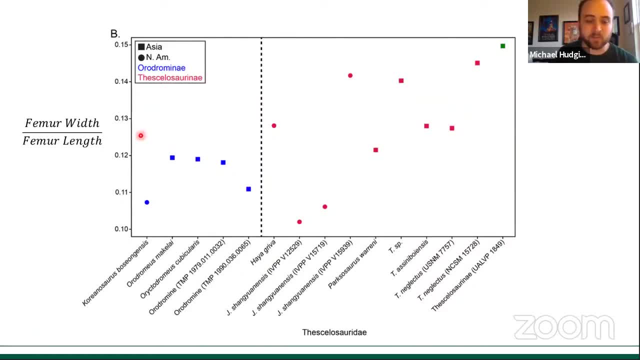 ratio of a femur width over femur length to see how robust the animal is, how robust the femur are. And so in the Y-axis we have the ratio here and in the X-axis is different. Thessalosaurid taxa. 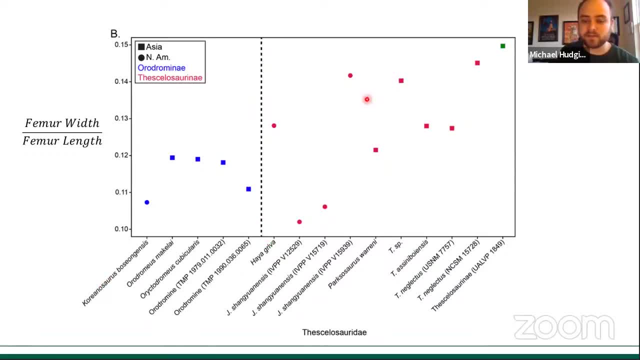 And the dotted line separates out Thessalosaurids from Orodromines. Orodromines are blue, Thessalosaurids are red, And Asian taxa are represented by the square and North American taxa are represented by the circle And the green is the DC bone bed, Thessalosaurid, As you see here. 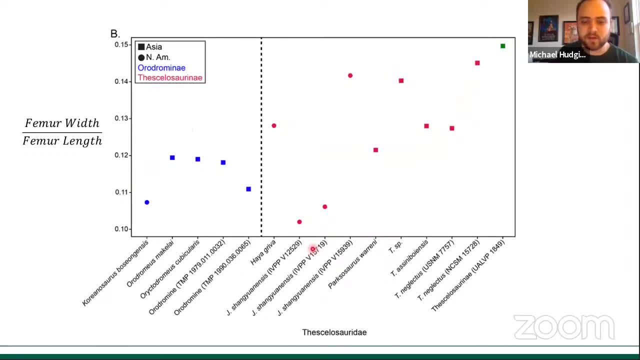 Thessalosaurids are fairly more robust compared to Orodromines. The two Jeholosaurids- Jeholosaurus are here- are representing a juvenile specimen and the adult specimen is here, So overall the Thessalosaurid taxa are fairly robust compared to Orodromines. 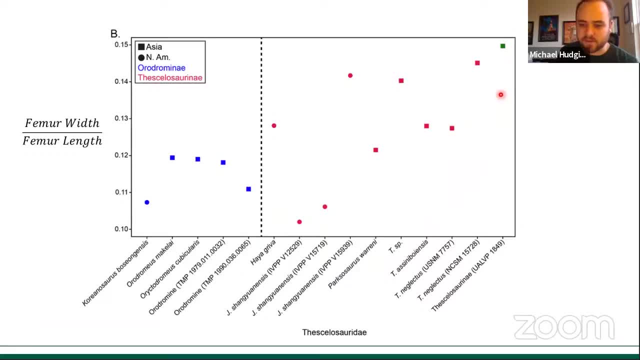 But the DC bone bed is more robust than Thessalosaurus neglectus, which is quite astonishing given that it is very small compared to Thessalosaurus neglectus. But it has overall a much more robust morphology compared to other Thessalosaurid taxa. 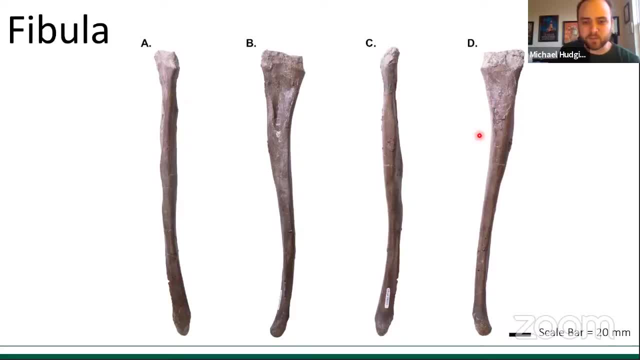 So the fibula is pretty typical of a Thessalosaurid. They have a lot of morphological features that are in common with it. It doesn't appear to be a ceratopsid or a hadrosaurid, because hadrosaurids and ceratopsid fibulae are fairly robust compared to this. They're just 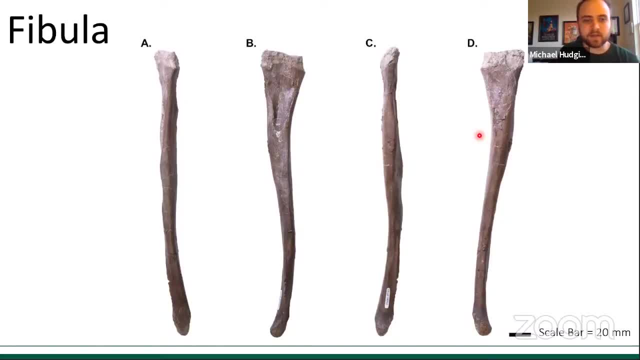 overall more bigger And it does not look like a Pachycephalusaurid based on Stegosaurus, where the fibula is fairly splint-like. It reminds me of a chicken fibula. It's just very small and it doesn't extend all the way down to the ankle, unlike the fibula of this Thessalosaurid. 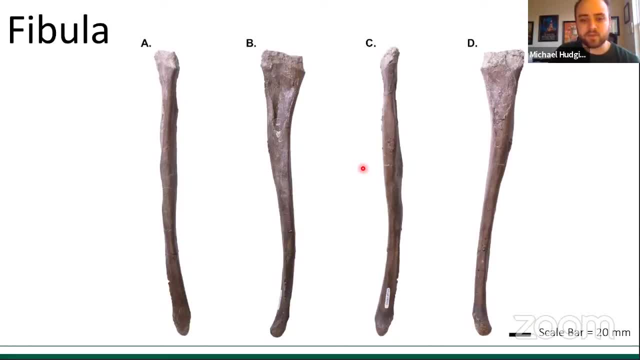 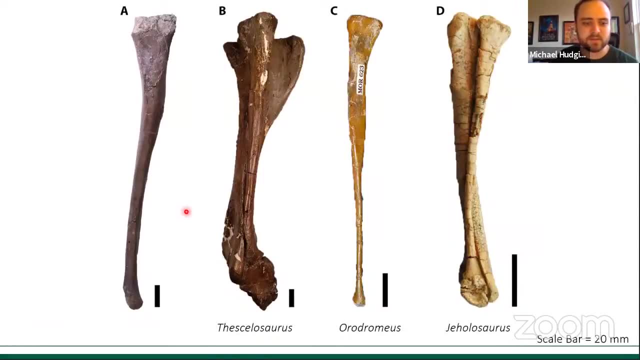 and Thessalosaurs in general, But when comparing with other Thessalosaurid fibula, it looks fairly similar to Thessalosaurus neglectus. So here's the DC bone bit Thessalosaurid fibula. Here's Thessalosaurus neglectus, or Dromaeus fibula, and Jeholosaurus. 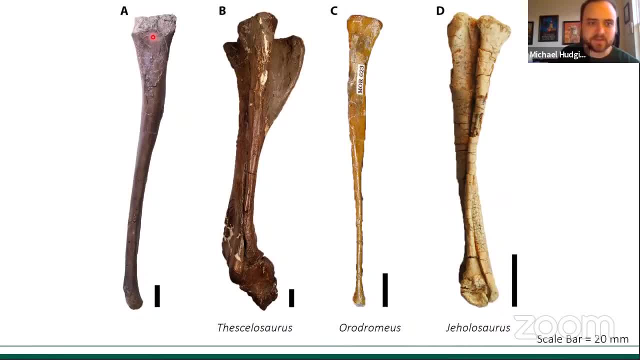 As you see, it looks fairly similar to Thessalosaurus. It has this kink right here. that's similar right here And it has this: Thessalosaurus has a slight sigmoidal shape compared, which is pretty similar to the DC bone bit one, as it has a sigmoidal shape here. 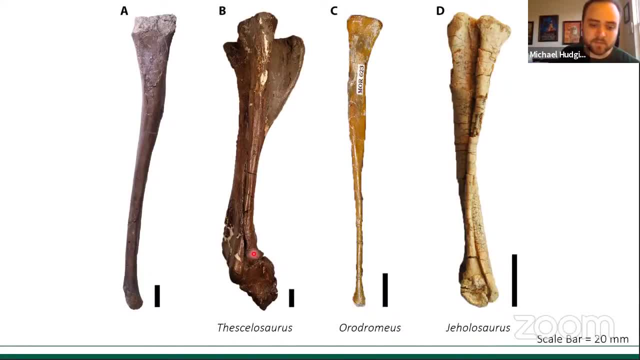 So if you follow this, here's the end that is touching the ankle of Thessalosaurus and it curves up and then almost forms a sigmoidal shape which is very, very similar to the DC bone bit Thessalosaurid. 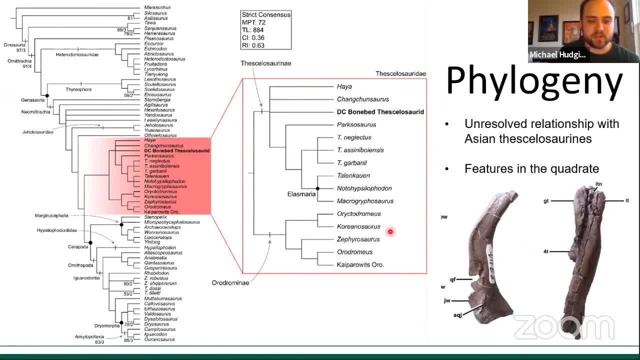 And so when I was doing the description and the comparative work at the end of it I was fairly convinced that it was some form of Thessalosaurid. whether it was an orodromine or a Thessalosaurian I was not able to discern based on comparative work alone. 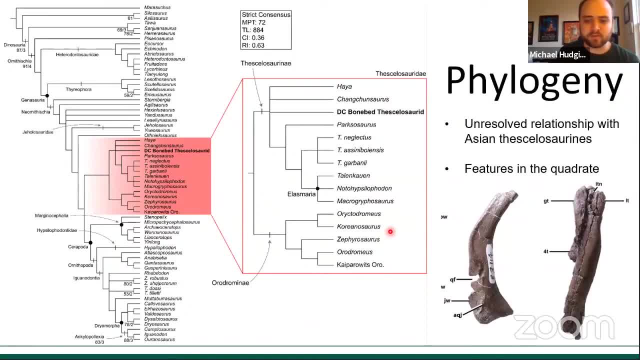 But when I inputted it into a keratin matrix by Boyd 2015,, the DC bone bit Thessalosaurid appeared to be fairly close. it appeared to be within Thessalosaurinae but forms a polytomy. 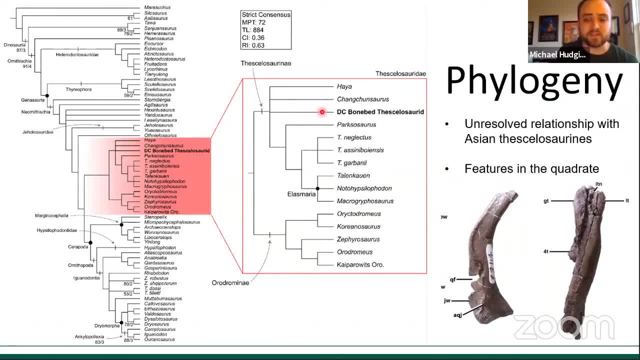 or an unresolved relationship with other Asian representatives, such as Changchangsaurus, as well as Hayek. So the features that diagnose the DC bone bit Thessalosaurid are features in the quadrate as well as the femur and it appears that they are fairly closely related to the Asian representatives. 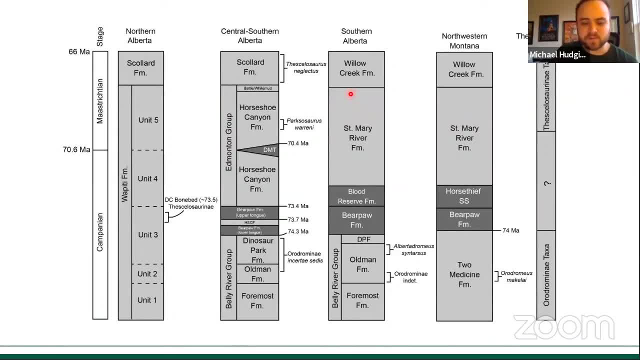 And so with this we can get somewhat of a picture of what's going on during the late Cretaceous, during the bear paw formation in southern Alberta, As this fossil taxa represents that missing time period in Thessalosaurid evolution. As I said earlier, the orodromine taxa occur in younger sediments in the Dinosaur Park. 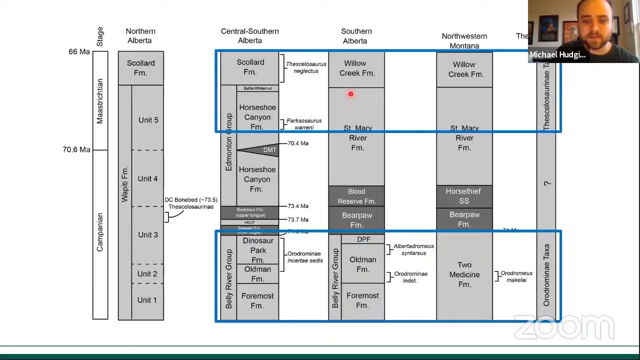 formation, old man formation and so forth, and Thessalosaurians occur in younger formations such as the Horseshoe Canyon formation and Scallard formation, And so it appears during the bear paw formation or during bear paw equivalent times. 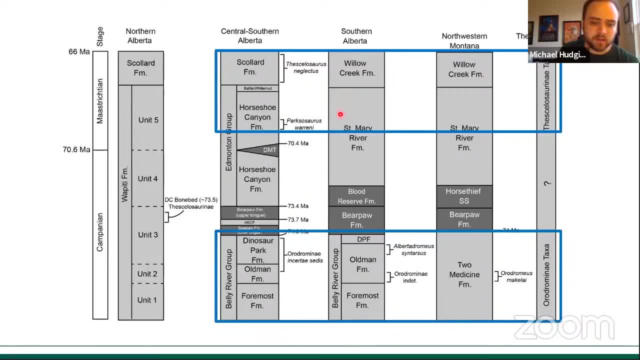 in northern Alberta, Alberta, is that thessosaurines were present during this time period. Whether or not that orodromines evolved into thessosaurines- probably unlikely, but the fossil material probably represents an Asian migration into North America of thessosaurines. potentially. 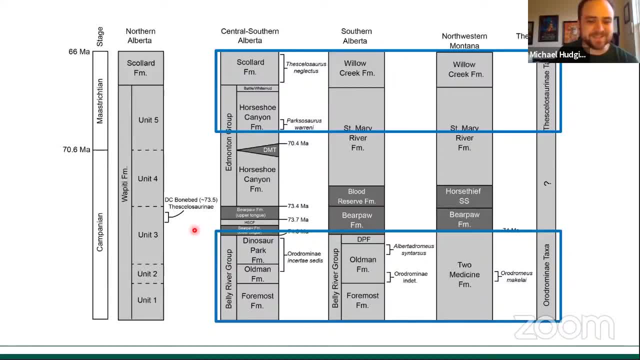 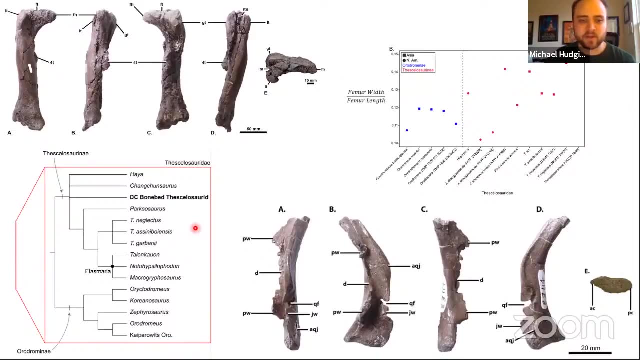 But more fossil materials is needed to figure out this problem of thessosaurid evolution in the late Cretaceous period, as you see here. So overall, it seems that the material coming out of the DC bone bed is a thessosaurid and more closely related to thessosaurines. 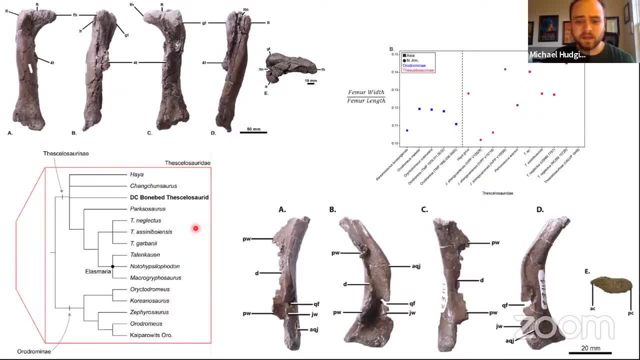 Asian representatives, such as Changchangsaurus and Haia, as features present in the quadrate, as well as the femur. And as well as the femur, is quite robust compared to other thessosaurid taxa as it has the most robust features- femur width over femur length- of any thessosaurid. 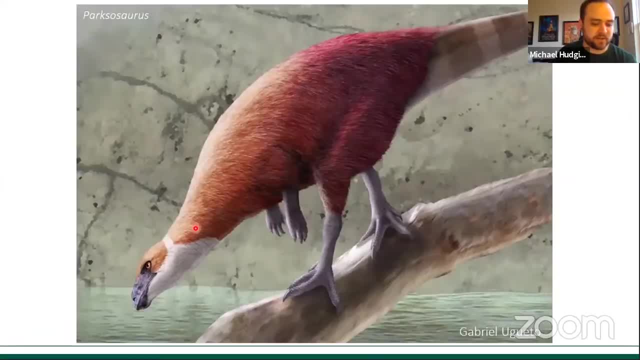 And so with this, thessosaurid evolution and thessosaurid research is pretty important because these animals represent kind of a hidden diversity during the late Cretaceous period, in which they probably make up a large percent of the ecosystem, during that time period. 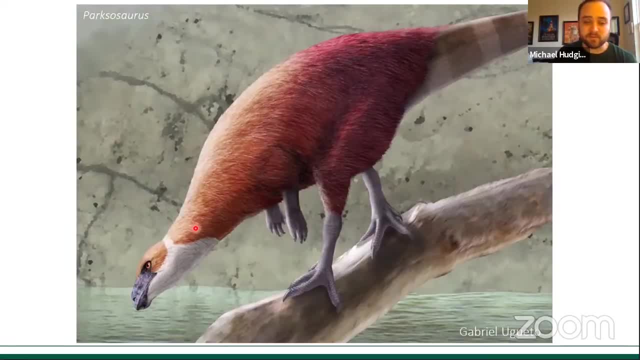 because they are small-bodied, But we really don't know much about their evolution, or nor do we know about their paleobiology. We don't really know much about their morphology, their individual variation between different individuals. We don't really know about their. 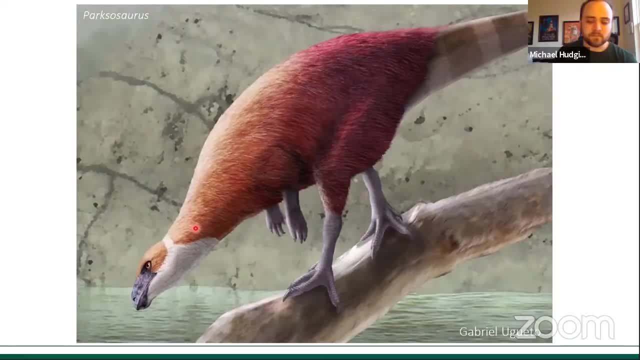 ontogeny and let alone we don't really know about their evolutionary relationships amongst Ornithischia in general. So with this, the DC bone bed is a fairly important find for thessosaurid evolution and paleobiology because it represents a thessosaurid in a time. 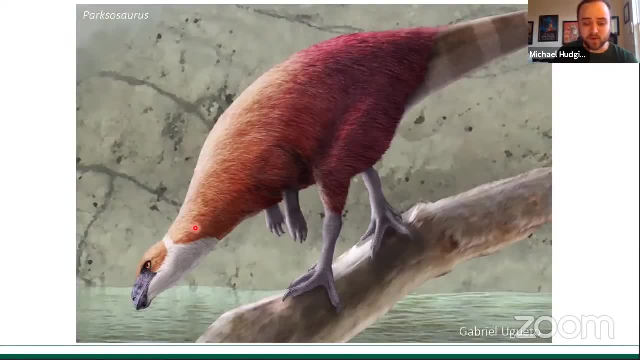 period that has not been identified. So we're going to go ahead and take a look at some of the species that have not been documented or been described, and we really didn't know much about this group of animals during this time period. and this fossil specimen elucidates the evolution. 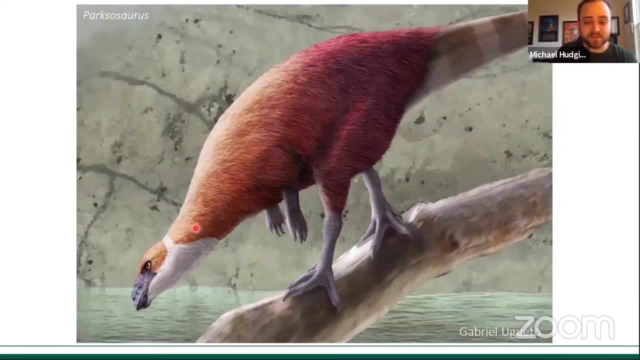 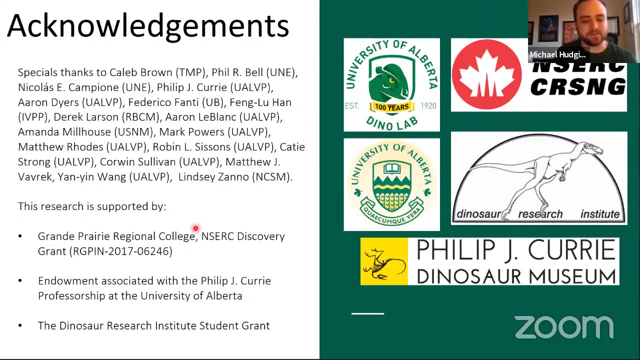 and paleobiology of this group. So here is Parxasaurus taking a bow, and I want to thank my research sponsors, as well as people who have helped me with this project throughout my master's school, And so I want to thank Corin Sullivan and Phil Curry for this project and being inspirations. 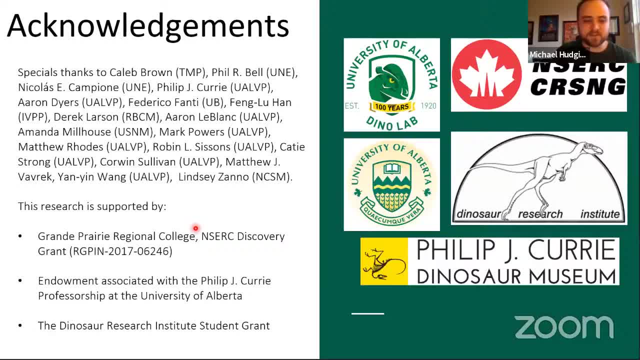 and as well as the grants from the Grand Prairie Regional College, as well as an endowment from the Phil O J Curry Professorship at the University of Alberta, and as well as the Dinosaur Research Institute student grant for allowing me to travel in weird times to look at specimens. 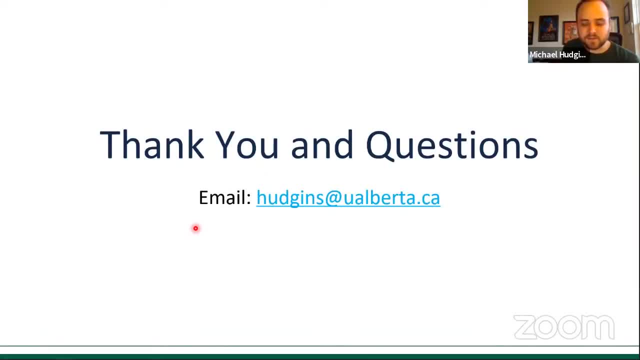 At this point in time I can take any questions. If you have any questions, feel free to ask them in the Q&A box below, And you know I would welcome any questions And thank you for having me. Thank you, Michael, That was a great talk. So yes, we are going to move into the question period. If anyone has any questions, just type it in the chat. 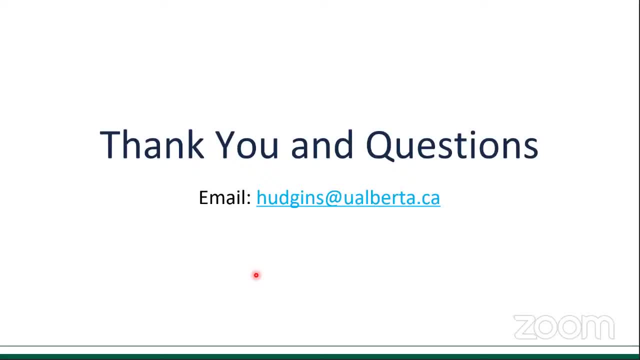 Our first question: What is your favorite dinosaur? Oh, I can guess and give the cliche answer: I like Tyrannosaurus Rex, but Thesajaurs have been growing on me so I really like Thesausaurus neglectus at this point in time. so I would say: 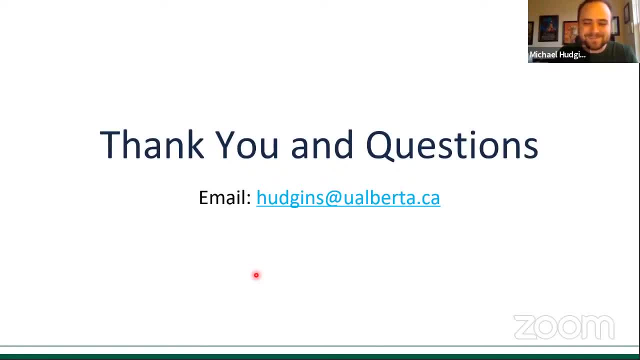 in time. So I would have to say Thesaurus. Of course That's a great dinosaur, as you just showed us. Yes, All right. second question: What has been the best advice you've been given in paleontology and who gave you the advice? Oh man, I'm kind of put on the spot for this one. 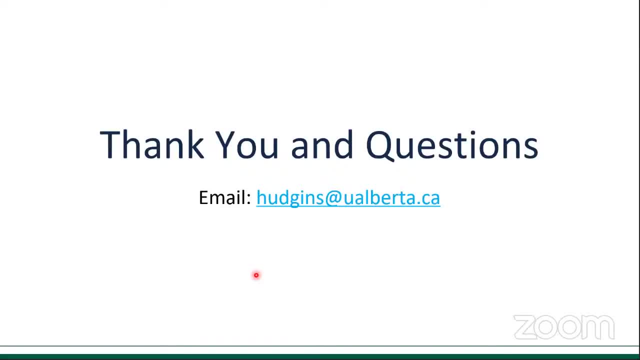 I don't know. Do you have any advice you'd like to give to somebody Looking to paleo, Getting to paleo? Never give up your passions and always be curious about the world. I think that's one of the best advice I can give, because a lot of paleontologists 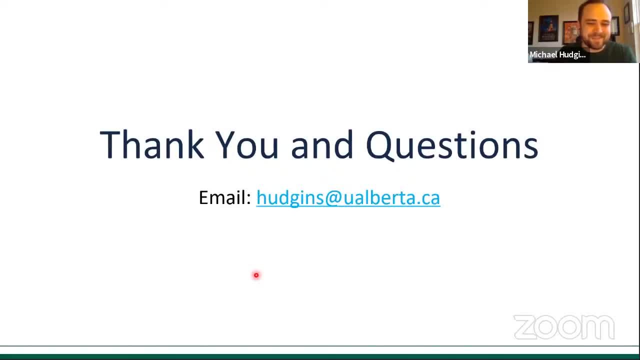 from my experience and what I've done, it's like we never really grew up. We still like dinosaurs- and so I still like dinosaurs- and never lose that intuition and that curiosity about the natural world and find your passion. I guess that's the best advice I can give at this point. 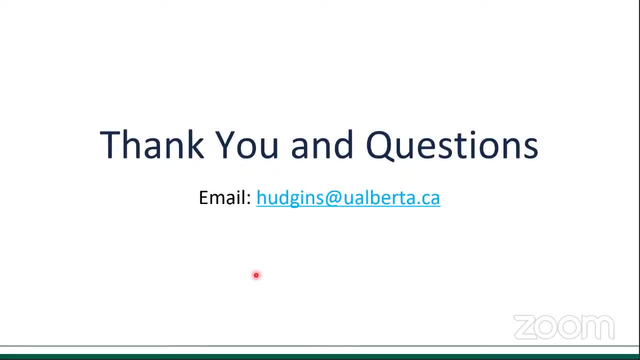 Beautiful, All right. next question: Are there any features in Thesaurus' skeleton that indicate that it burrowed? So with Orodromius- well, Orodromians in general, in previous studies from Vericchio et al, and I think, one of his students, Farallon, 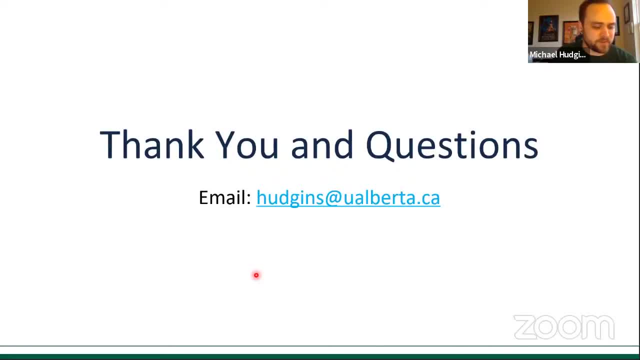 and he was the advisor. they were looking at morphological features within Orodromius that could be diagnostic to a burrowing behavior, And they found that the scapula was fairly different from other Thesosaurus as well as from other Ornithischian dinosaurs And morphological 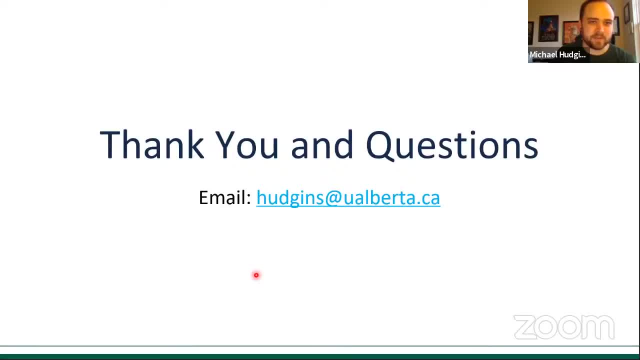 features that would signify a burrowing type of lifestyle would be larger muscle attachments on the scapula. This was called the scapular spine, just for one example, And they linked that as a key characteristic. So yeah, that was one morphological feature, but yes, 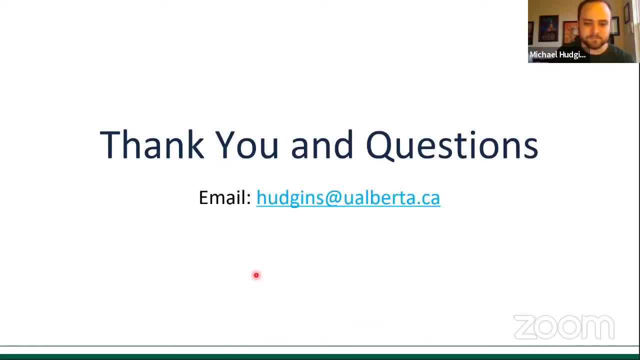 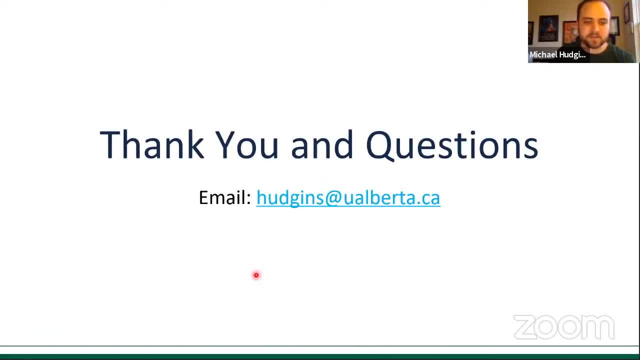 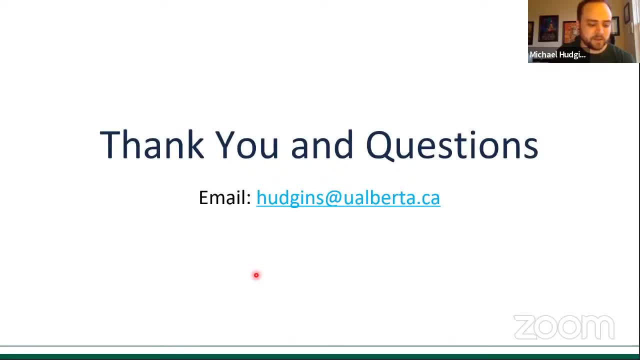 is all, I think, Maastrichtian in age. But the Parxosaurus tooth taxa might be up for debate because the tooth that was found in the Prince Creek Formation was a premaxillary tooth And we don't have any premaxillary teeth of those. 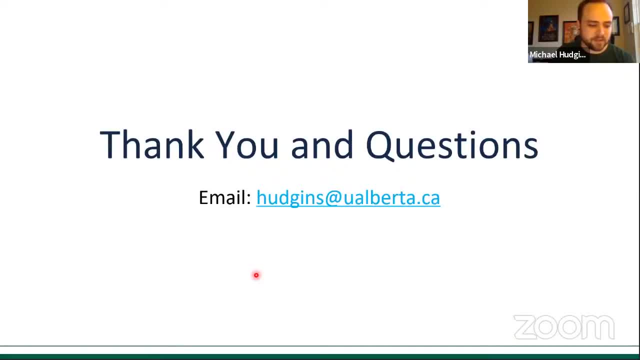 So when the researchers were describing the tooth, it looked fairly similar to Thesaurus, but not quite like Thesaurus, And so they kind of hypothesized or predicted that the tooth represents a Parxosaurus instead of a Thesaurus. But we don't really have a lot. 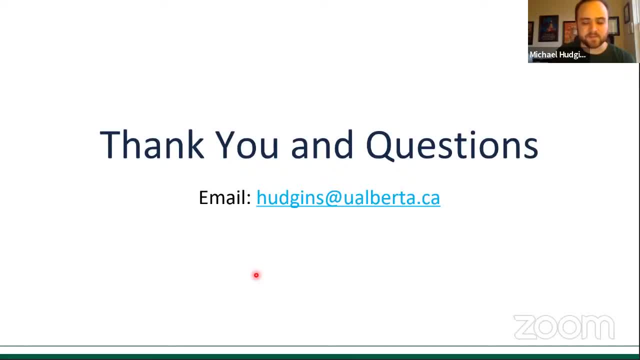 of fossils from Alaska. that represents a Thesaurus, I guess anybody doing paleontology in Alaska- keep your eyes open. Mm, hmm, all right, um, uh, your undergrad work- was it in biology or geology? um, so i got my undergrad in geology at george mason, and so, um, with paleontology it can go either way. you can either go in the 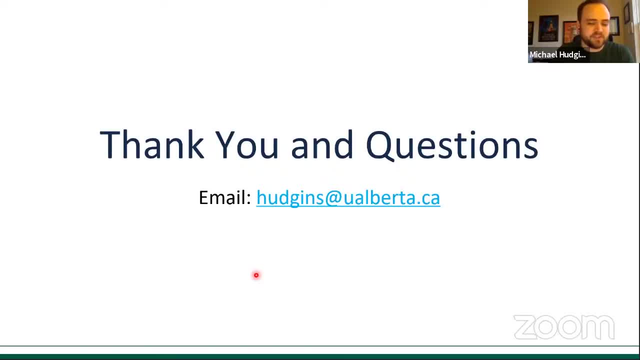 biological route or the geological route. i went the the geological route. i wanted to get that time context of it and understand where these fossils are coming from in the rock and interpreting what the rock tells you about the taphonomy or the environment which these animals lived in. 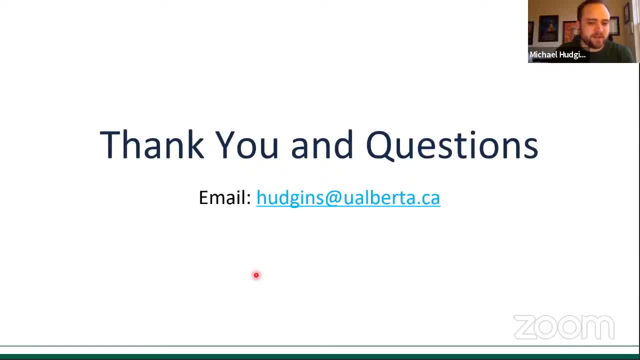 right, and so i. i got my geology degree, but it was concentrating in paleontology so i took a lot of upper level division of biology, of biology classes that coincided with my geological studies. next question: uh, will the dc bone bed theslosaurus, get a new name, since it could be diagnosed? 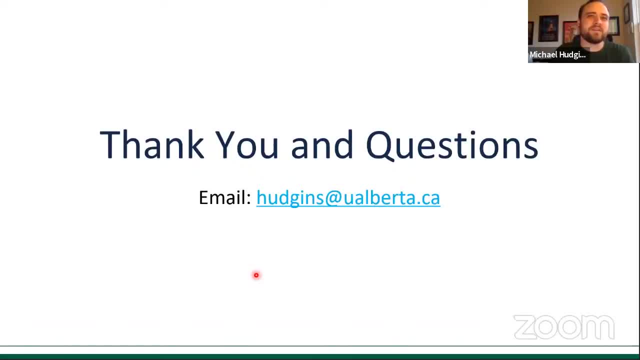 um, i don't think so. one, because the material is fairly fragmentary and unassociated, as well as there's not a lot of. there aren't really any diagnostic features within this material, other than the fact that the material, the femur, is fairly robust. but i don't think it's. it's good enough to name it a. 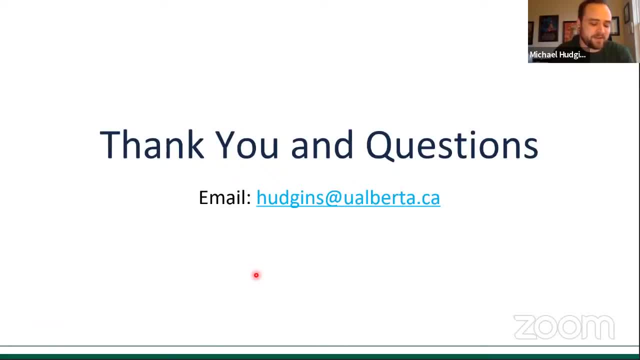 new taxa, but it is interesting and there might be a new theslosaurus in the uh, in the wapiti formation during that time frame, um, but more fossil material is going to be used to name it, you know, but that has been approved by us and the uh, the theslosaurus, disentangling. 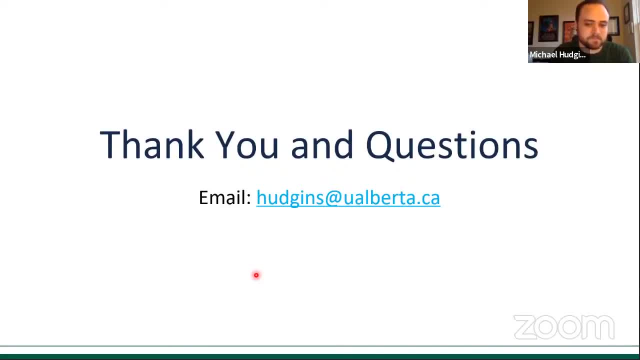 em persecutors. we believe that can be understood as a detectable Mon athlete development. so that's that's a really good question that could be used in a in a same Eatam field. yeah, so i guess this is just the current semi-ex WOODRUFF. 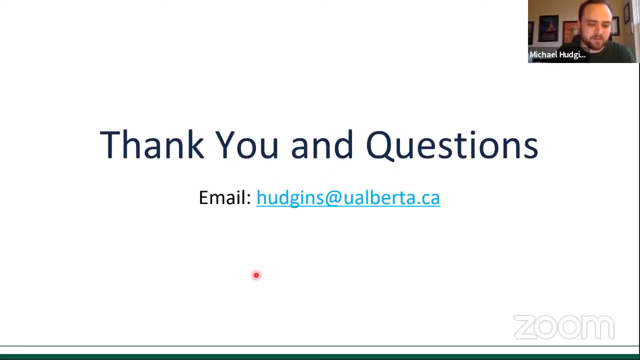 screw-shaped burrow-like structure in the rock, And so they found adult specimens as well as juvenile specimens in the burrow, And so that's what made researchers think, oh, this animal might have burrowed, And it also probably took care of its young in the burrow as well. based on the 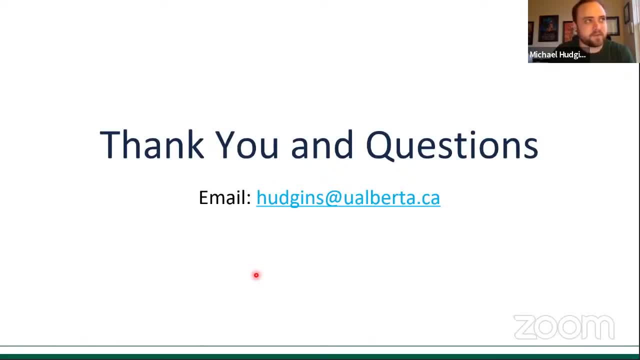 fossils that were present within the structure. So yes, there are igneofossils for burrow structures, Especially, I think it's only in Eryctodrome. yes, On a related note, what is your dream fossil to discover? 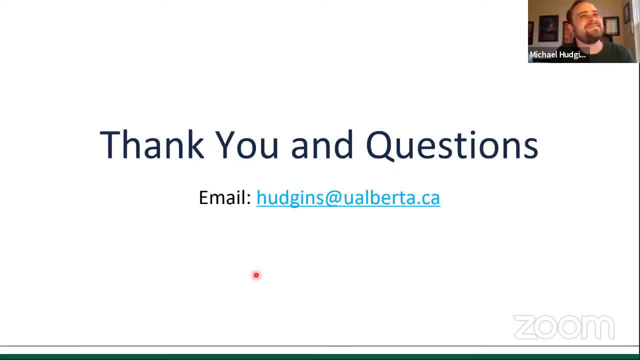 Oh, a Thessalosaurid type fossil that's sitting on a nest with a bunch of, with a complete ontogenetic sequence, A complete growth series, so we can understand their, their nesting behaviors and their morphology, their variation throughout their life. I think that would be an ideal fossil. 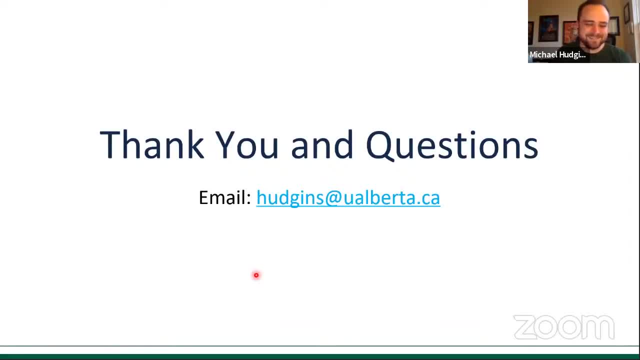 but that's very, very unrealistic. You can always keep your fingers crossed, Yep. Where have you done field work and where would you like to do new field work? For the most part it's been mostly in Alberta, mostly northern Alberta. 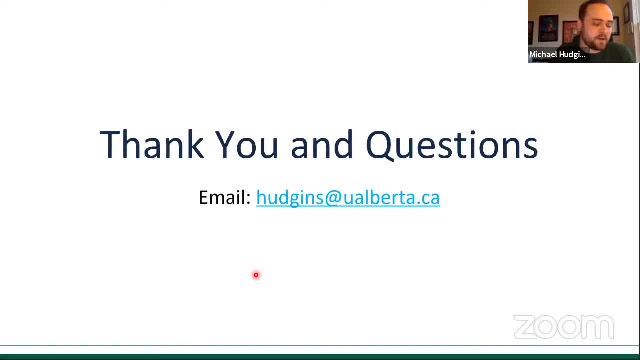 but I've done field work in Yorktown Virginia as well, and also in southern Virginia. When I was in undergrad I was invited along to excavate an American mastodon. I was at St Charles University, but that's, that's down in Yorktown Virginia. 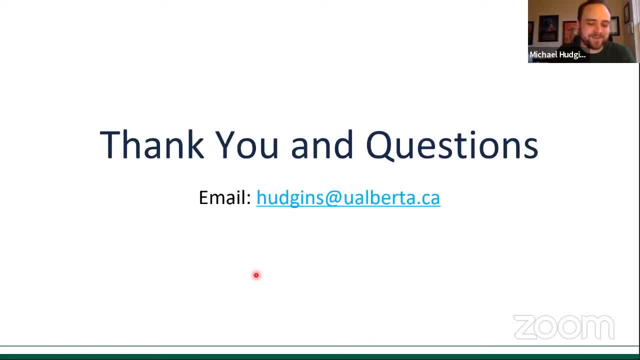 which is kind of kind of funny that it was about a mile away from my house in Yorktown at that time, and so I was invited by one of my geology professors and he took me along and uncovered a mastodon. so I thought that was pretty cool, but most of the field work is in Virginia. 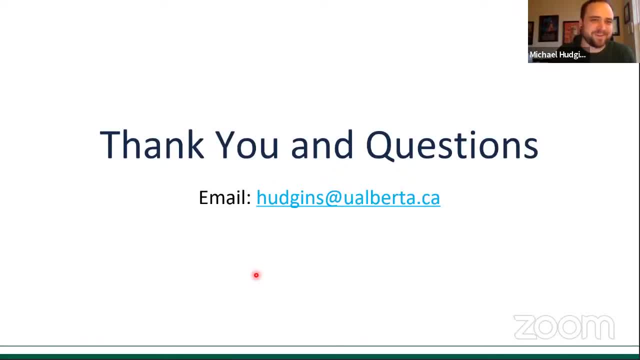 was in Virginia and northern Alberta, but I would really like to go to Mongolia. I really really want to go to Mongolia to do some fossil collecting and also go to Mongolia, and I think it's a really really cool thing. 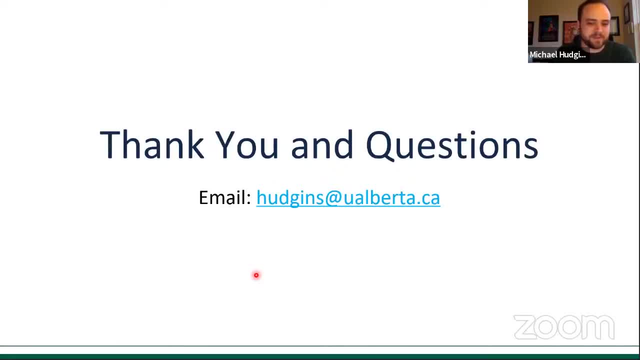 and also going to the collections at the museum and the capital, Mongolia, to look at some specimens. So Mongolia is my preferred choice right now. That would be very amazing. If you had your choice to research any topic in the future, what would it be?